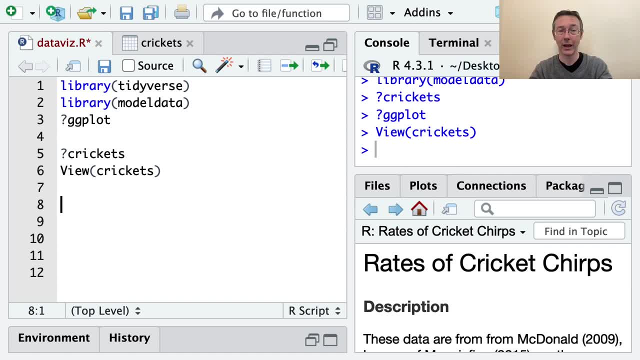 x-axis, the y-axis, are they using color size or something else? We specify these things first and then only specify the exact kind of plot, scatterplot, histogram, etc. later. I think it's easier to see than to hear. So let's get our first ggplot call. We only have one function. 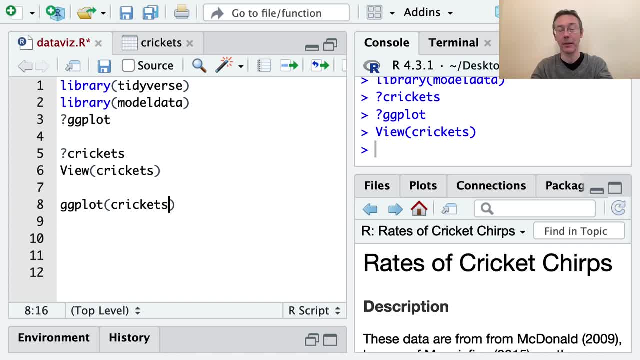 for plotting most plots in R, and that's ggplot. The first argument is just the data set crickets. If you're trying to do a plot that's not using a data set either, you're not really wanting to work in R. R, specifically, is for working with data. 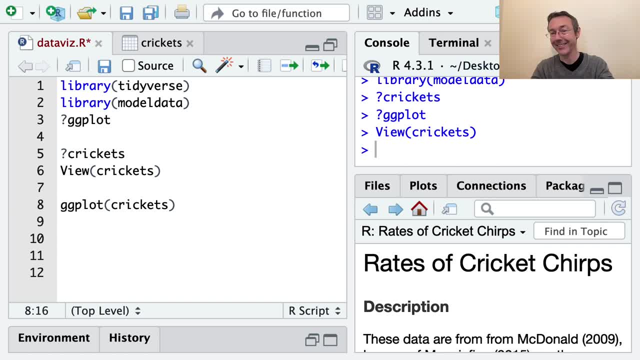 or you need to do a little pre-processing first to get the data in the right format, to get it in a data frame format. This goes along with the tidyverse idea that we should separate out our data preparation from our data visualization. Okay, the next thing we need to. 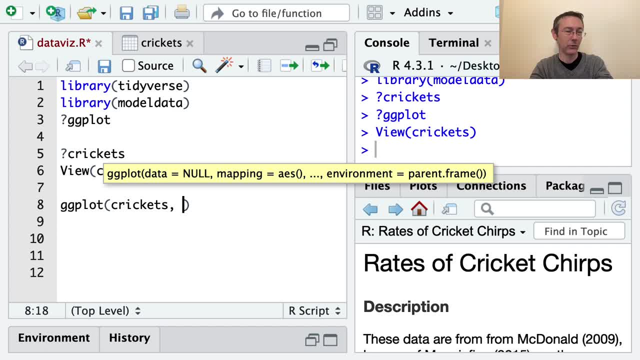 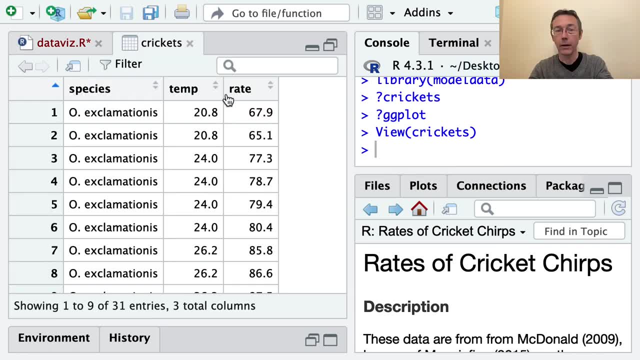 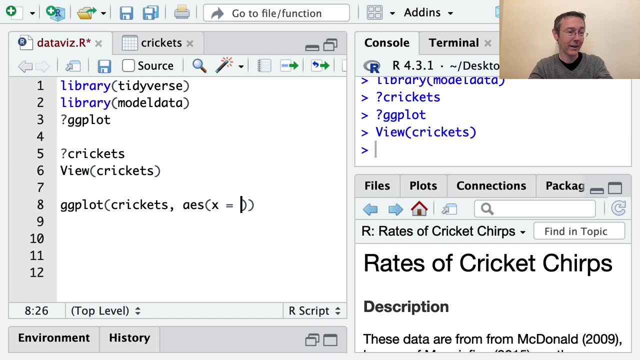 specify in our ggplot call is which variables are in the plot. So if I'm going to do a scatterplot, which variables are being displayed where. So if I want a scatterplot of rate versus temperature, I want the rate on the y-axis and the temperature on the x-axis. So I specify within the aesthetic: 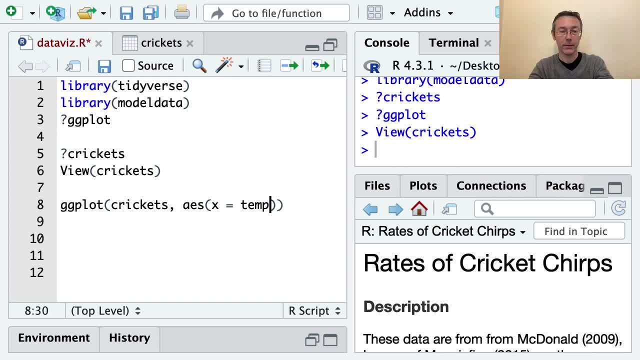 AES I say x equals temp and y equals rate. So how are those variables being mapped to the actual visualization? How are they going to be displayed? Okay, now that I've specified which variables are in the plot, I can specify what variables I want where it's time to actually tell R how to display. 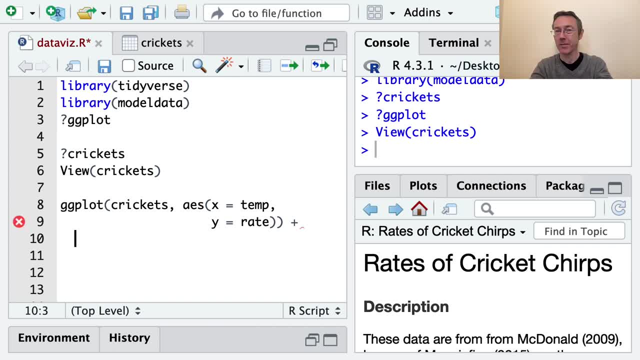 the data, In other words to tell R that I want a scatterplot, And I do that by specifying geom point. In general we specify the sort of plot we want, with plus geom underscore, and then the type of plot. So we'll later see geom histogram, geom bar and a few others Here. geom point: 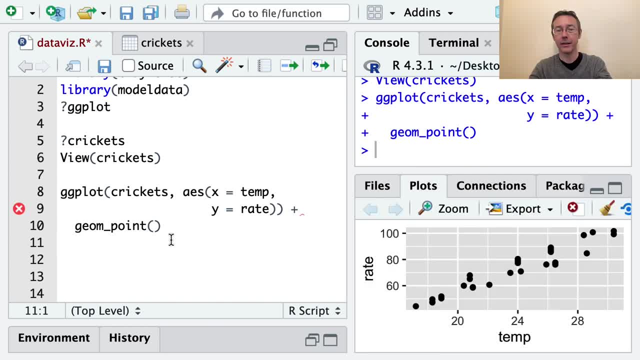 So for a basic scatterplot that's all I need, And if I'm going to do a scatterplot I'm going to hit command enter. We can see that here in the lower right. I'll zoom in on it to make it a little. 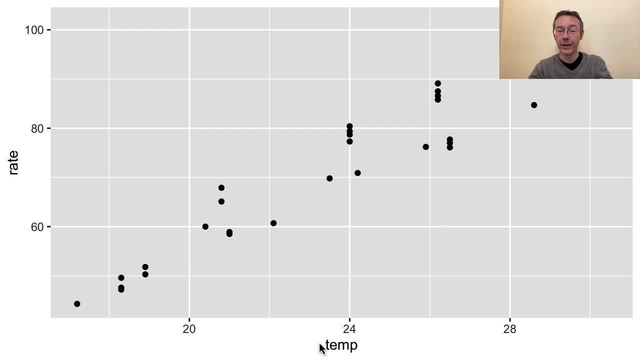 bit more clear. There we go. Notice that temp is the exact name of the variable, the exact name of the column that we are plotting. Rate: same thing. So the labels have been put in automatically using column names And then for each row in the data set. now we have a single point on the plot. Great. 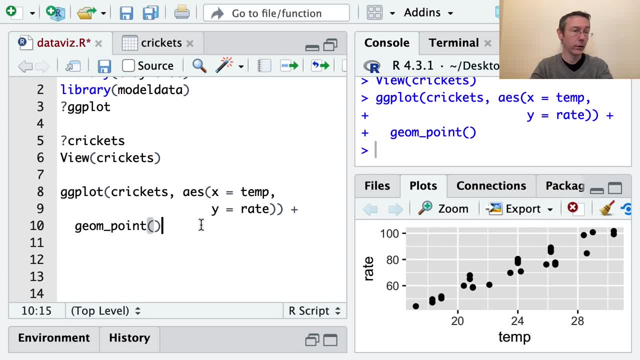 So there are any number of things we can do. We can do to improve or change the appearance of this plot, And the philosophy of the grammar of graphics and ggplot2 in particular is that those sort of non-data aspects of the plot, 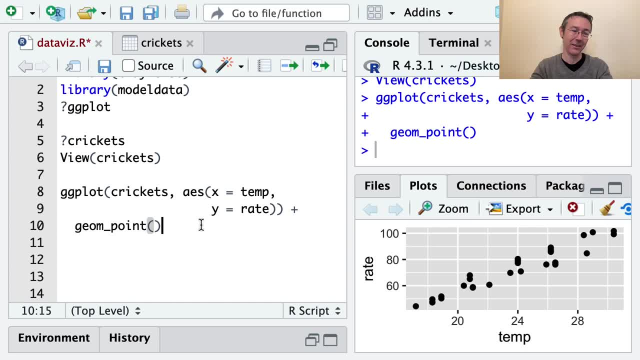 should be handled separately, after we've got the basics of it down, after we've specified the data set, the variables and the geometry, the geom, For instance, to change the labels we do plus labs, Self-explanatory the name of that one. 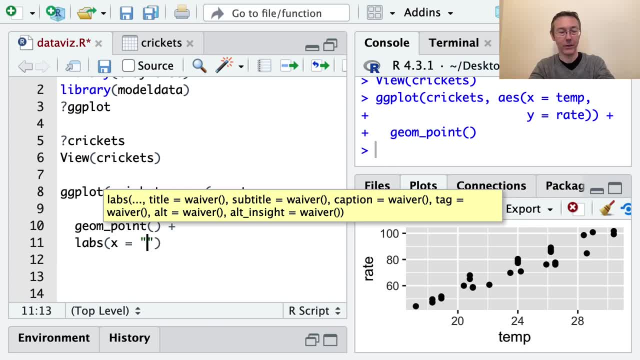 And then we have to say what we want the label on the x-axis to be. So in this case, how about I capitalize it and put temperature, And on the y-axis I'll put rate. Maybe I'll put chirp rate. 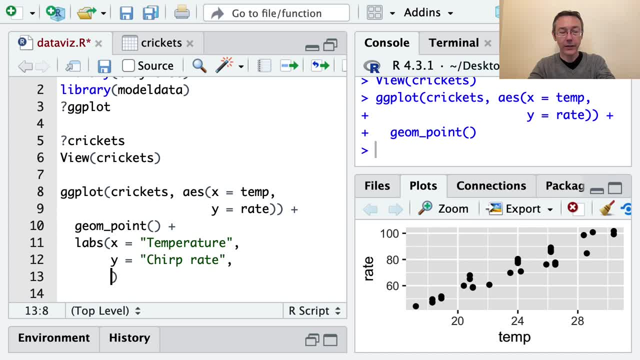 There we go. We can add a title. Let's do that. How about crickets, Cricket, chirps? We could add a subtitle if we wanted. I don't think I'll do that. We can add a caption, a caption like that. 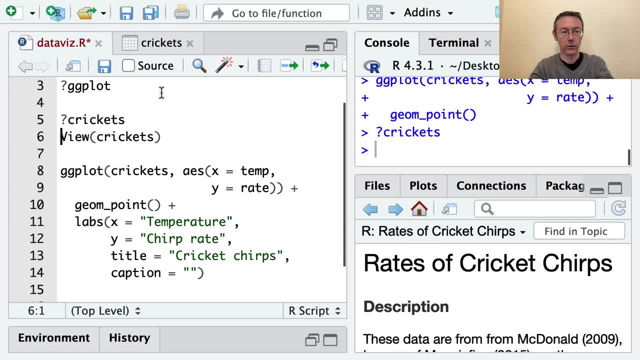 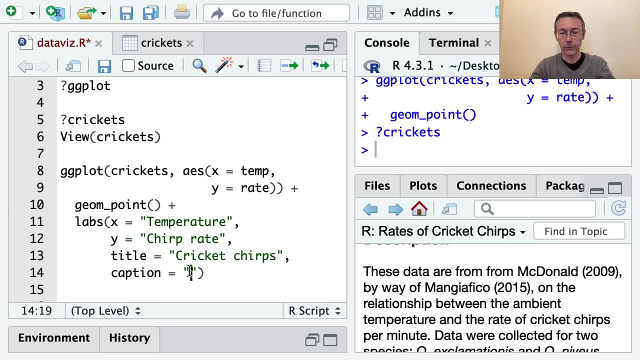 are often nice to cite your sources, so in my help file question mark cricket crickets, i can see a citation for mcdonald 2009.. for the moment i'll just put mcdonald 2009. if this were an actual plot for publication, i'd probably be a bit more descriptive than that. 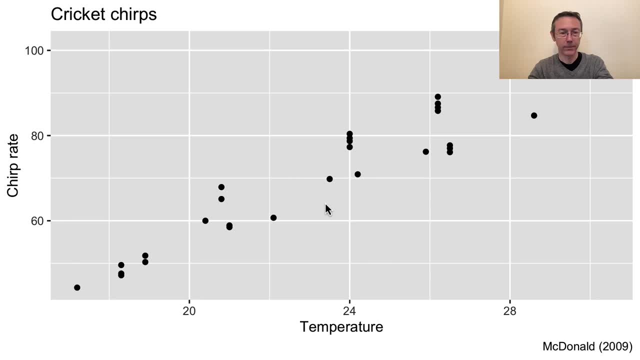 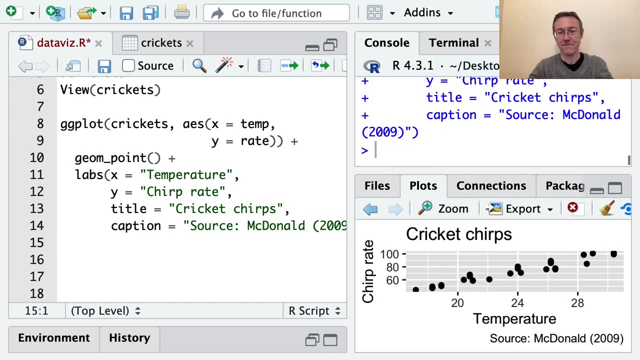 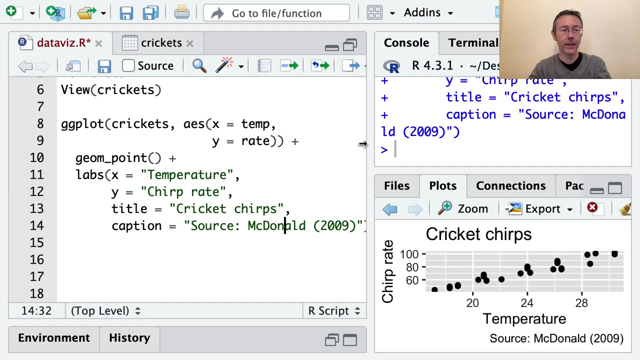 okay, so now you can see the title of the plot and the source. i think i actually want to label that. that is the source, so i'm going to label that as mcdonald. there we go, so that looks a little better, okay, so, um, there's lots of other aesthetics we can use. in this case we said we wanted to plot temp. 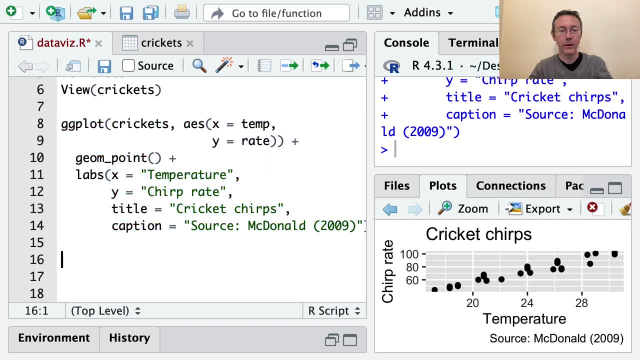 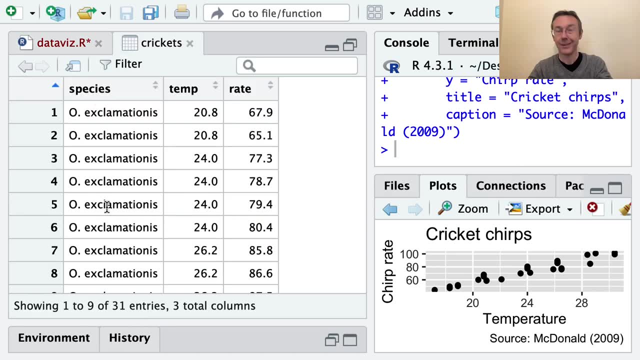 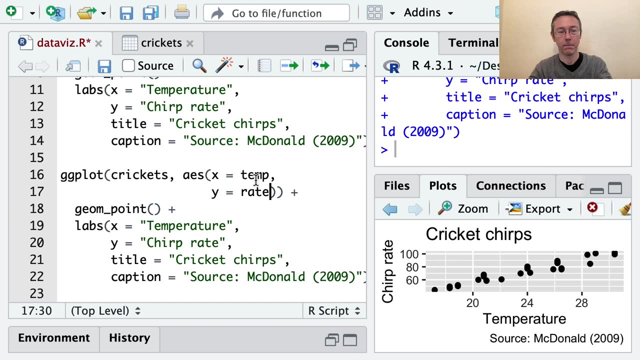 and rate on the x-axis and y-axis respectively. um, what about if we want to color this by species? so what i'm saying is that the species variable should be displayed in this plot. i want to map the species variable onto a color aesthetic, so i'm just going to add color equals species inside of my ggplot. 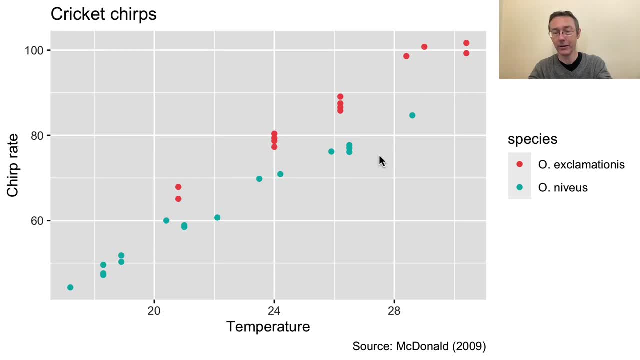 and if i zoom in you can see that now i have two different colors. here i have a legend on the right that went in automatically. i'm not in love with the fact that everything else has a capitalized letter at the beginning. here i do not. i want to change that label as well. the labs: 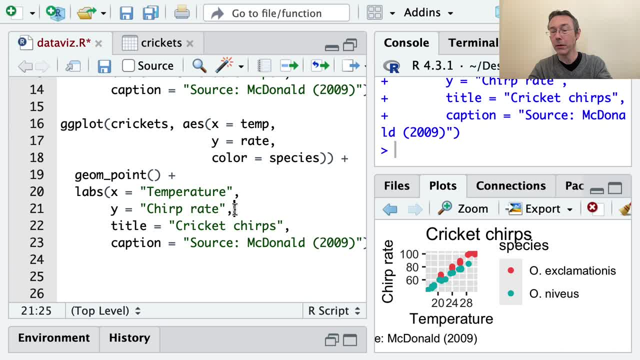 command here changes can change- can be used to change the labels on the color aesthetic in exactly the same way that it's used to change the labels on the x and y aesthetics. i just do color equals. quote capital species. and there we go. you can see that now, species in my legend here. 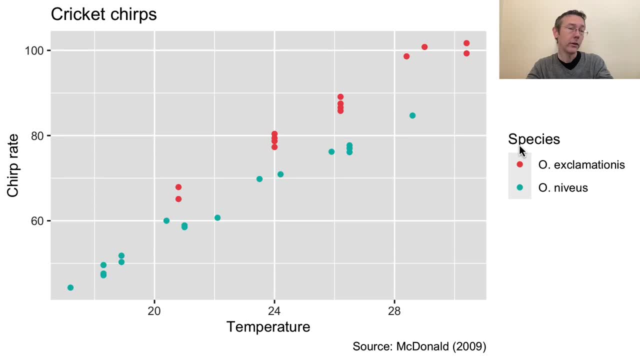 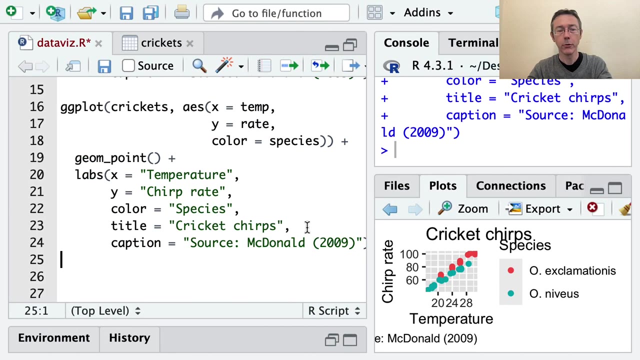 is capitalized. one potential problem with this comes in. if you are color blind, you may not be able to tell the difference between these two colors here. The default color palette in R and ggplot isn't great in that way. For improved accessibility I recommend this line of code that: 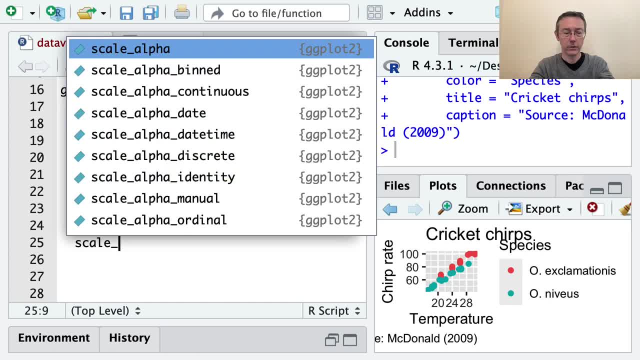 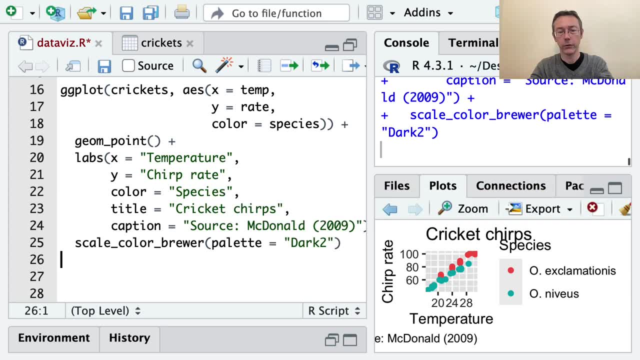 I won't say too much about It's scale. color brewer palette equals quote dark two and that'll change it to a slightly higher contrast, more colorblind, friendly palette Scale, because I'm changing the scale on a certain aesthetic Color, the name of the aesthetic, and then brewer is the 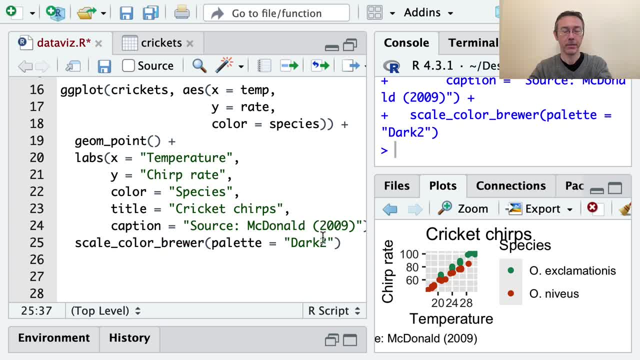 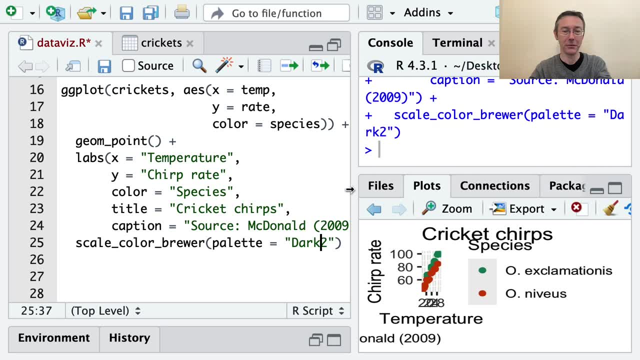 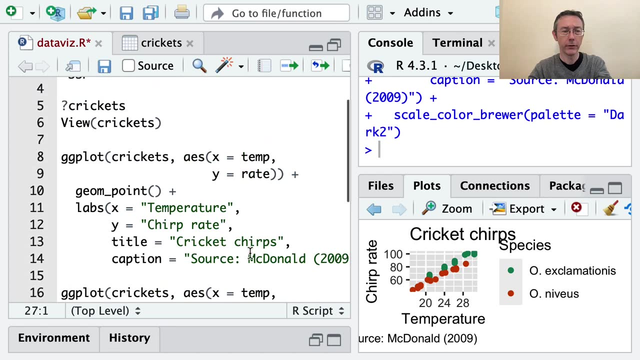 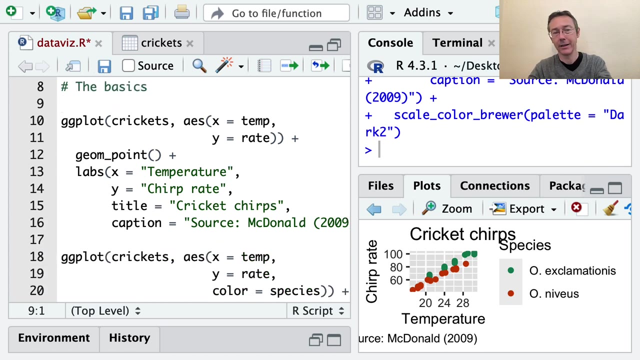 referring to the package from which this color palette is taken. So adding that on at the end of my line plus scale color brewer changes my color palette to something a little bit more friendly. All right, wonderful, Let's see here. Let's go put in some comments here. So I'll comment this one as the basics Doing a scatter plot. 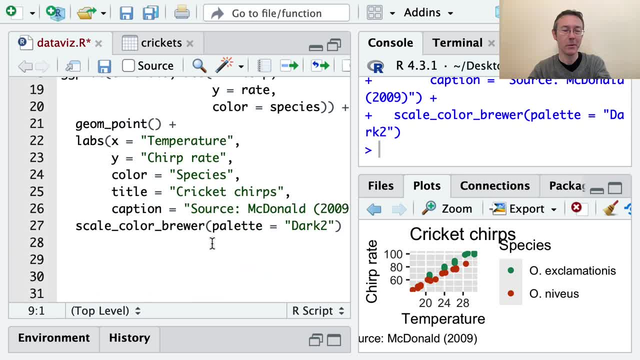 changing the labels, adding some color to it. Good basic stuff. Let's make some more modifications. I'm going to go back to this first one. I don't want to color it by species, just for this next few, these next few examples. 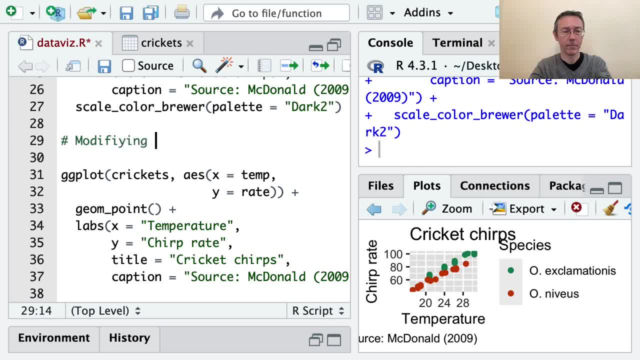 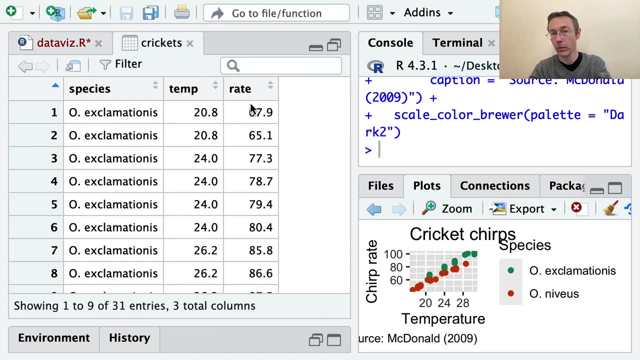 How about modifications? How about modifying basic properties of the plot? So we know now how to change or decide which variables are in are being represented in the plot and how those variables are being represented. But what if I just want to directly make a change? 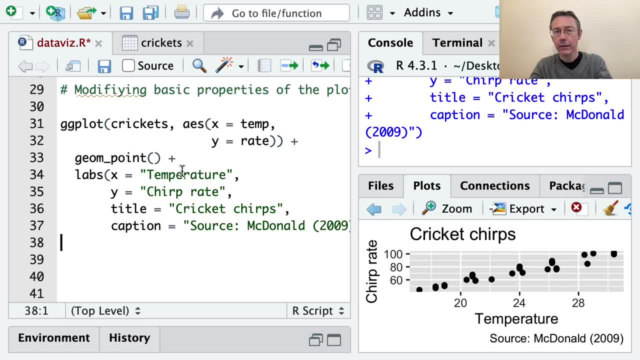 What if I want to take these points and just make them all red? I don't want them to come from a variable now. I just want to specify red. That's not an aesthetic. that doesn't go in here. Aesthetics tell us variables and 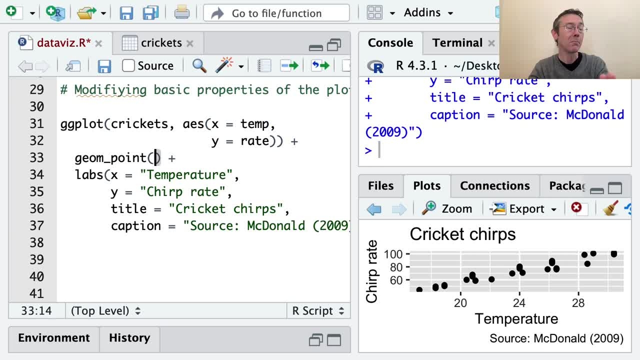 how they're being displayed. If I want just a basic property of the geome that goes inside of the geome, So for instance, to change the points to be a red color, it would be color equals, quote red. You can specify colors using hexadecimal codes. There's other ways to do that as well. 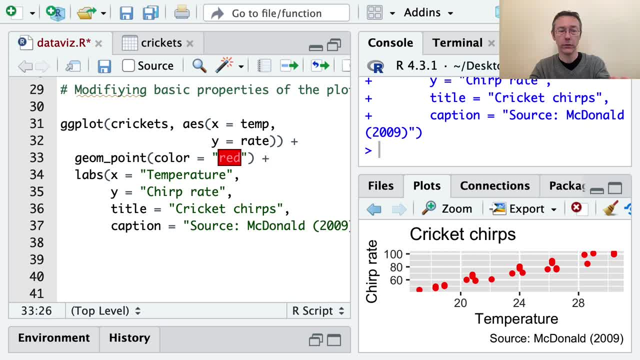 There's something like six or seven hundred colors that are recognized just by pockets, Period, just by name. So there's some interesting ones. There's like peach puff is one of them, That one's not a high contrast one at all. You can do gray. There's like eight different grays, or 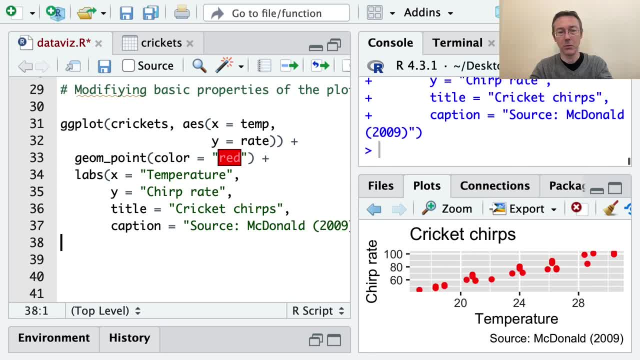 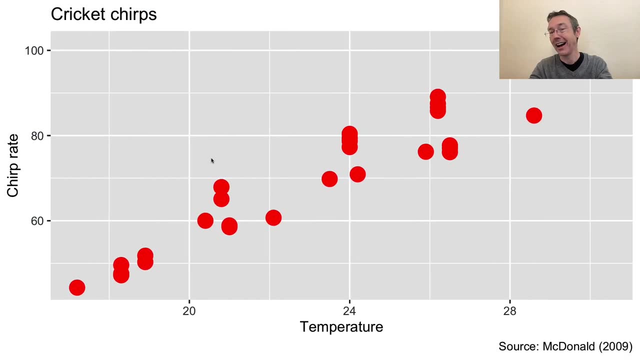 something. I think red was the most visible, so I'll stick with that. We can change the size of the points, For instance, we can make them larger. Size equals two. Sometimes you just tinker around with that, There's size five, for instance. So making them five times as large, I think I'll. 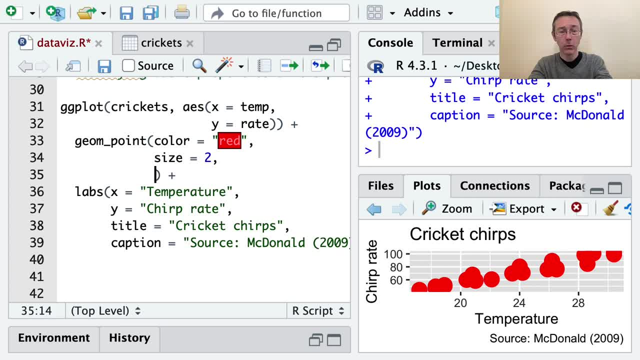 leave it two for now. Another thing I want to make you aware of is that you can change the transparency. If you add alpha equals and then you put in a number between zero and one, it'll tell you sort of how opaque it is. So I can make them 80% opaque with alpha equals 0.8.. Maybe I'll make. 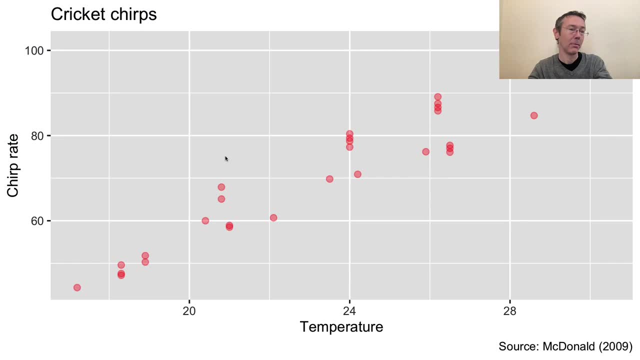 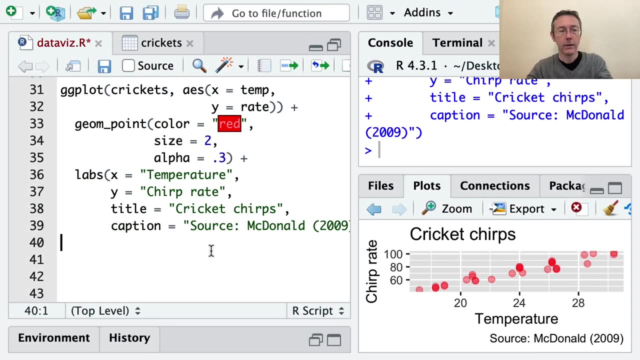 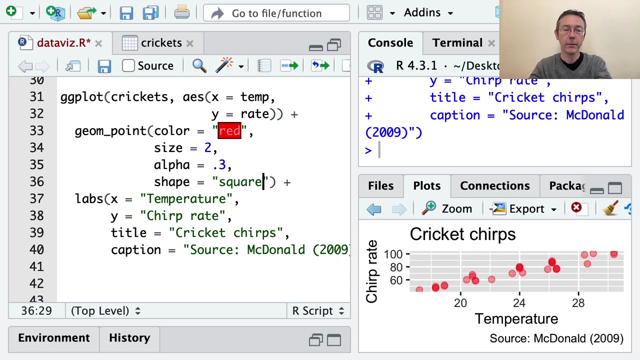 it, alpha equals 0.3, so that it's even more apparent from my plot. This is particularly helpful if you have potentially over-plotting. Okay, size alpha. One other thing you might want to do is shape. For instance, we can change our shape so that all 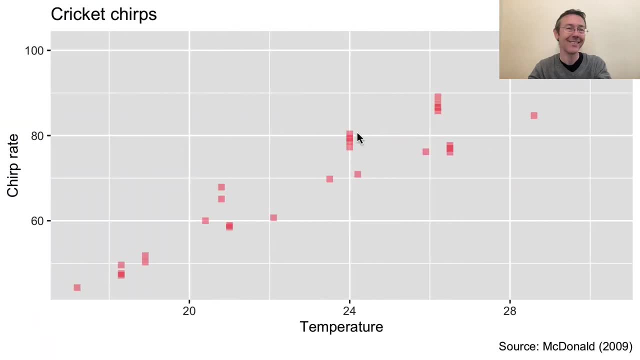 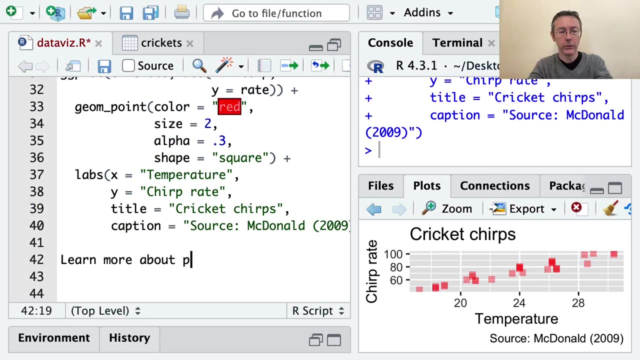 the points are represented as squares And you can see that pretty clearly here. Instead of the dots, I have squares. Learn more about the options for the geom. Oops, I need this to be a comment, Sorry, Just by question mark: geom, whatever. 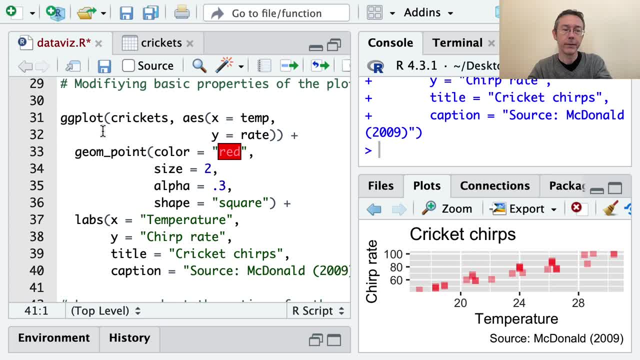 One of the really nice things about this structure for ggplot is there's not just a help file for ggplot, There's a help file for every single one of your geoms, like geom point. You can get the help file for labs. You can get the help file for ScaleColor Brewer, for instance. 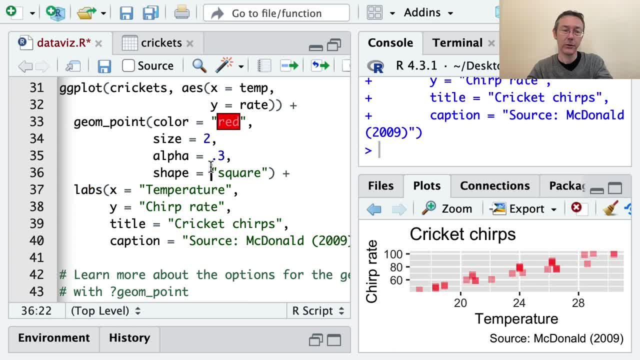 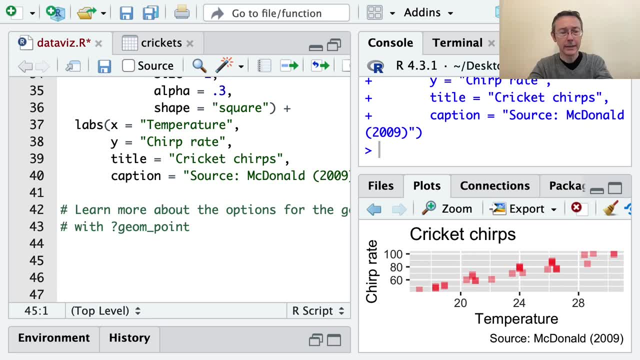 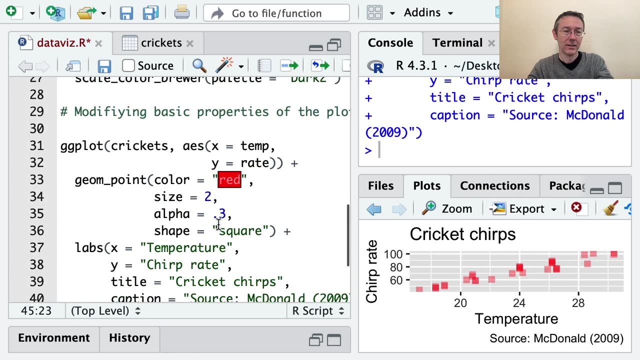 All of these things have their own help files, and that allows for a much higher degree of granularity and the kind of help that you can get. Okay, let's see here Adding another layer. Okay, so I'm going back to this first one again. 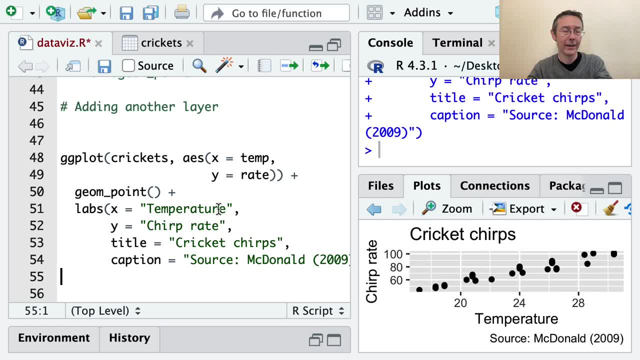 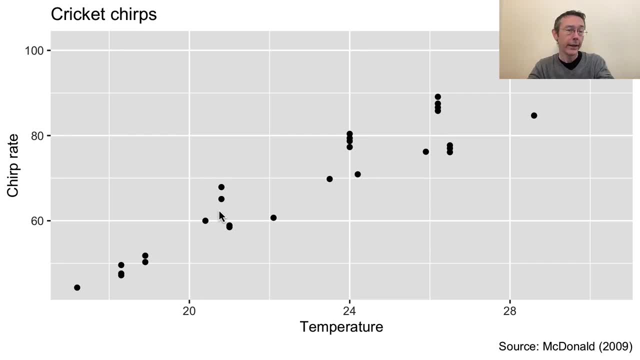 I'd like to put a regression line over this. This is a more or less linear shape. There's- certainly it's not a perfectly linear- relationship, but it's relatively close. That's just another layer on the plot. I still want to be using the x values of temperatures. 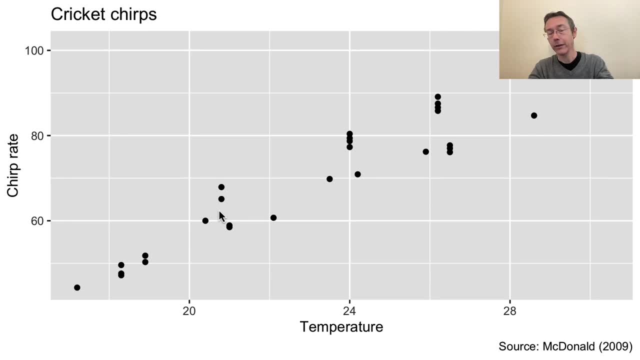 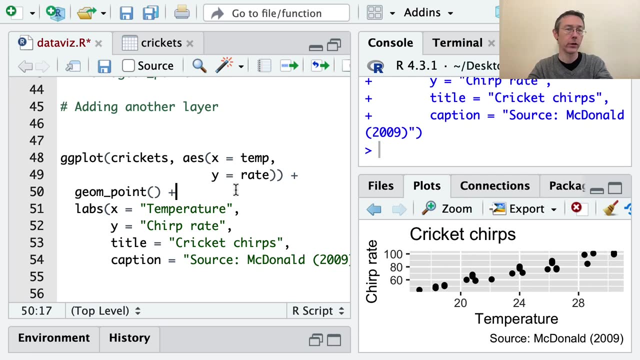 and the y values of trip rates as I calculate the regression line. One of the great things about ggplot: you can just add as many layers as you like. It's like you're working on a canvas painting: one layer, then another, then another. So after my geom point I will put geom smooth. 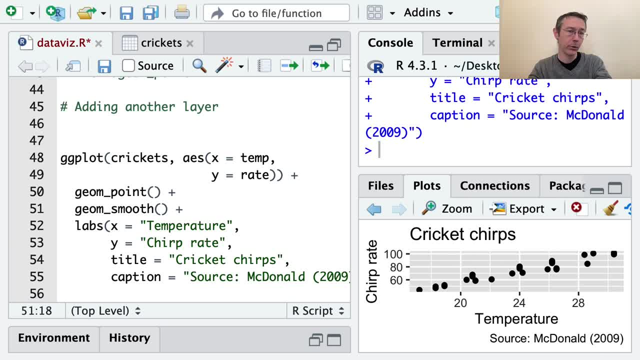 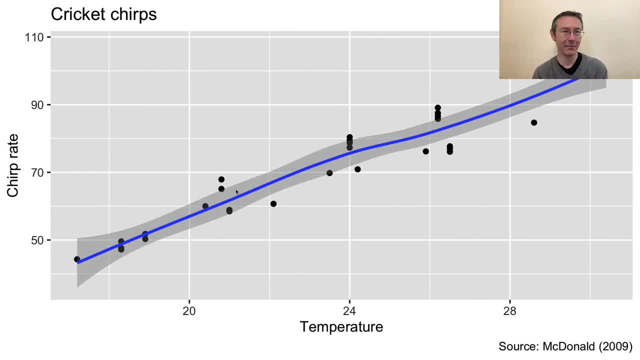 And for the moment I'm just going to leave it as is. It won't be a regression line yet, but that's okay. Okay so it's almost like a line, but if you look closely you'll see it's kind of a little bit squiggly. This is R's default way of fitting a smoother or a curve of best fit. 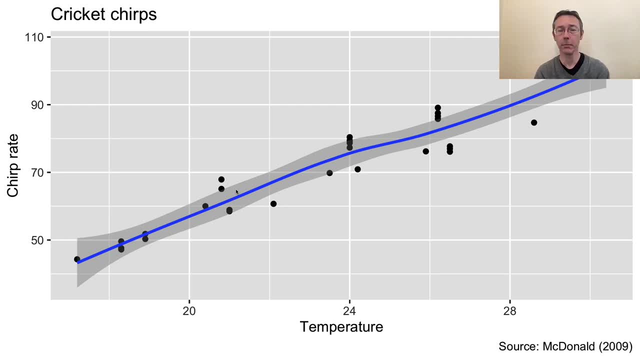 over the data. It's using a low S curve. that's kind of a rolling polynomial fit, not a regression line, So that can fit the data A little bit more closely and be a little bit more flexible as it captures the trend of the 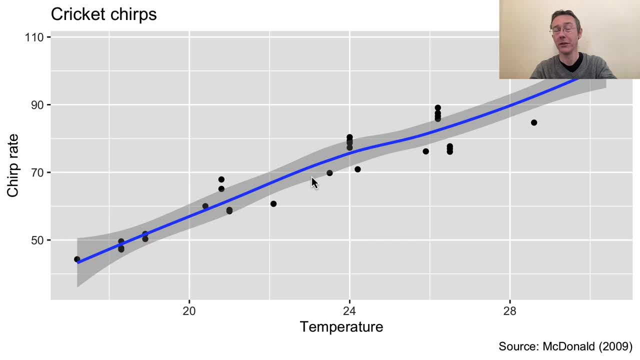 data, It's a little bit more opaque. There's not a simple formula for this. It doesn't contribute as much, maybe, to our understanding of the relationship between these two variables as a regression line would, So I want to go in and make this an actual line. 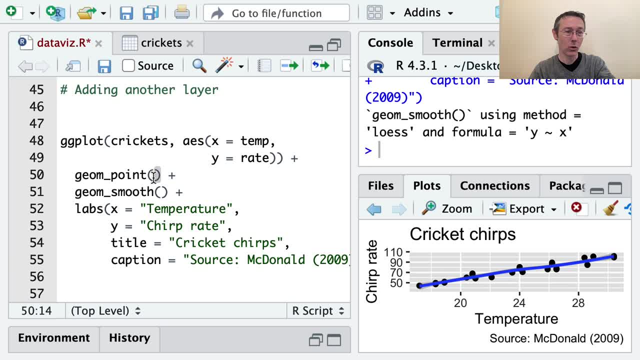 Just like I could add arguments to geom point to change the qualities of the points, I can add arguments to geom smooth to change the qualities of the smoother. In this case, I want method equals, quote lm, Use a linear model And of course I could learn more. 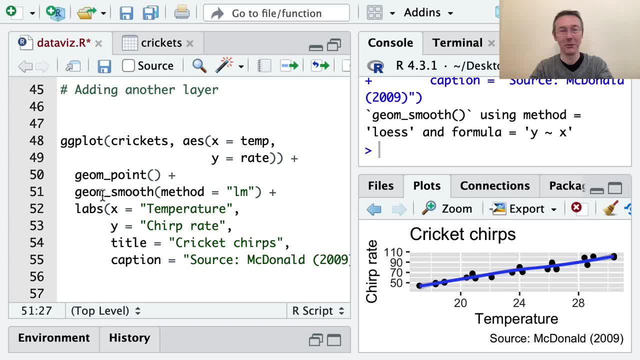 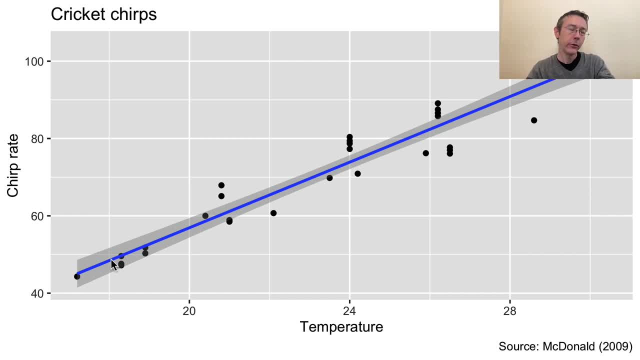 about how to do this with question mark geom smooth, and the help file would give me lots of good guidance on that. Now you can see it's actually a regression line. Notice the gray bar here, that error ribbon. That's giving us some measures of uncertainty in this regression line. 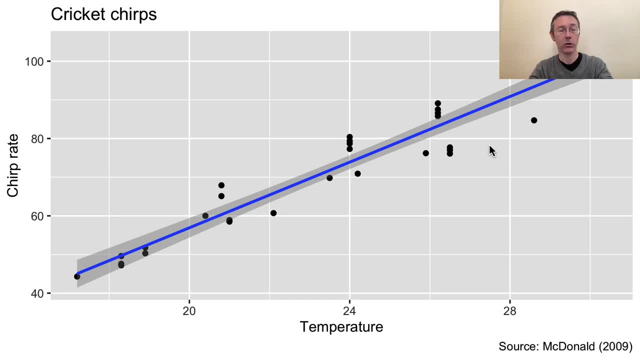 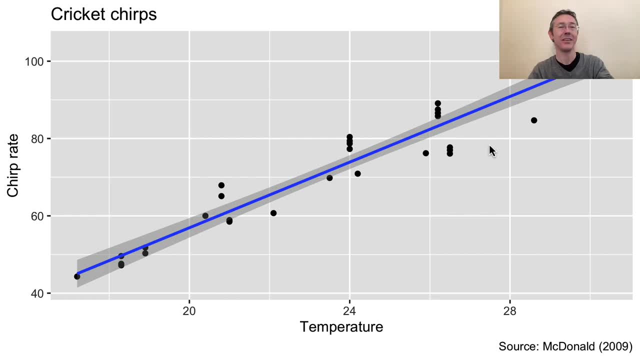 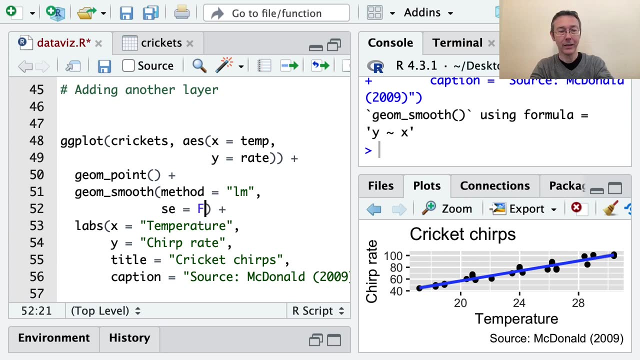 So I'm going to go in and see if I can do that. So I'm going to go in and see if I can do that. That can be helpful in some circumstances. In others it can just make the plot seem more noisy or busy. I'm going to remove it just to show how With se equals false. So se for standard. 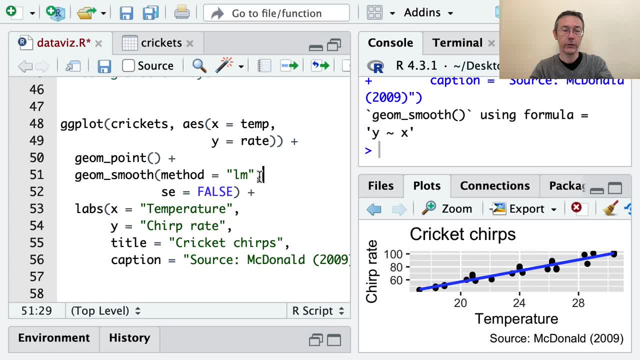 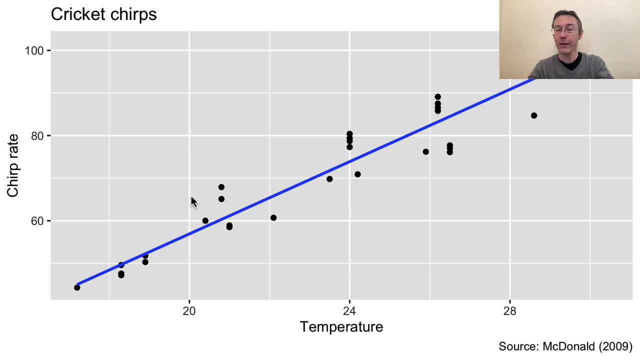 error. Take out the standard error ribbon. Notice that there's a comma separating the arguments. Notice it's inside of geom smooth, just like so Fabulous. So we've got a decent regression line for this data. Last thing I want to do on this scatter plot: 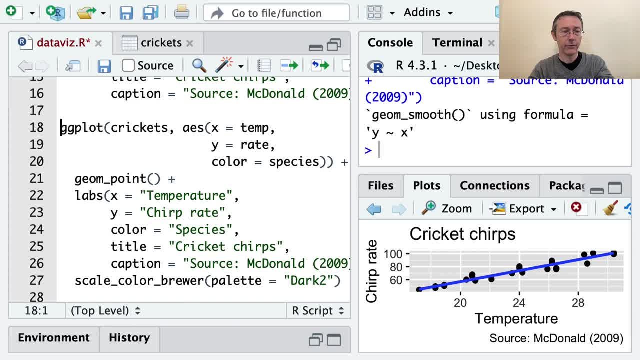 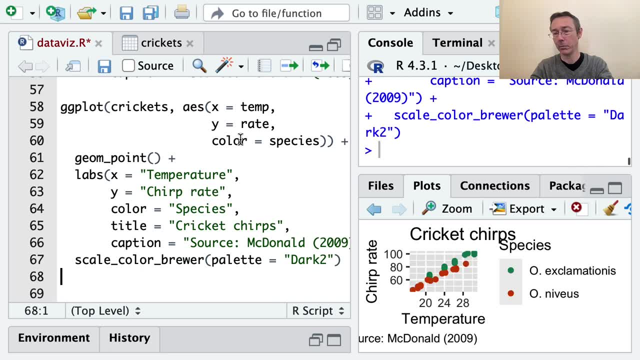 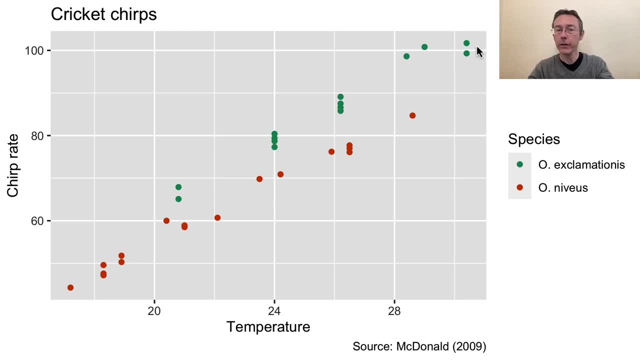 is point out, what happens if I do a regression line when I had added a color aesthetic. So, looking at this plot, Remember here I have each species with a different color And you can see that within each group we've got a pretty good linear relationship. In fact the non-linearity. 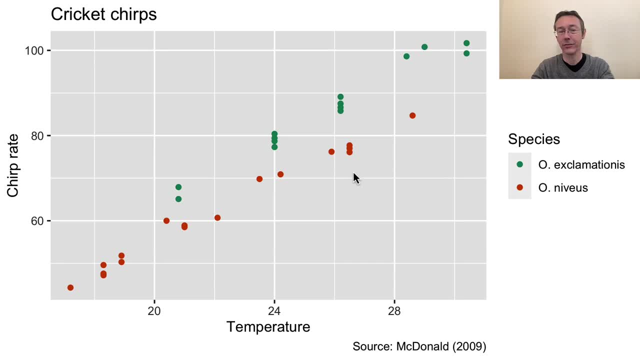 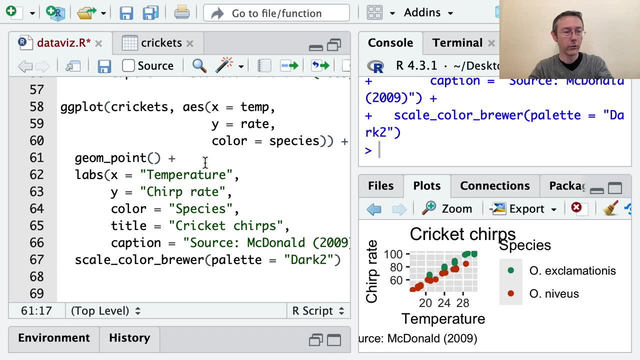 in the original plot is probably due to the fact that really there's two species here, each of which have a very linear relationship. Let's go to geom point and do, and after that add a layer that is geom smooth, And I will stick. 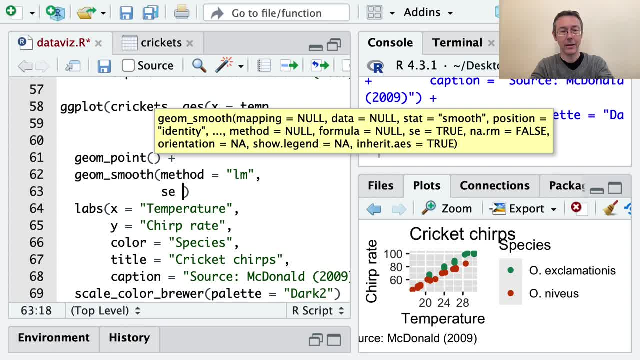 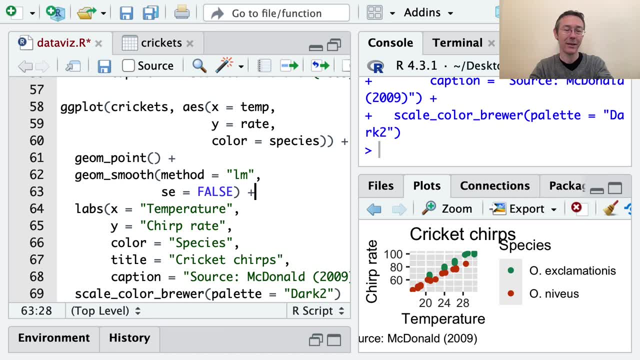 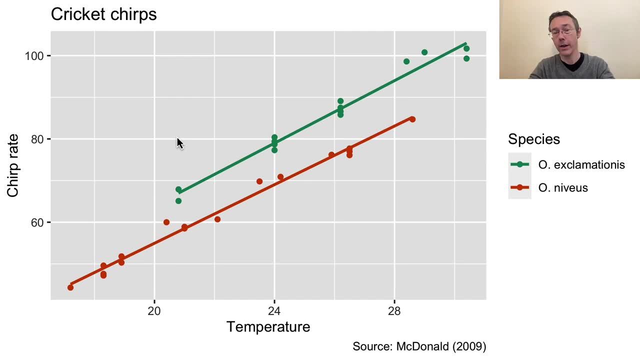 with method equals quote lm, so that it's a regression line, And se equals false, so that it is taking out the standard error ribbon to make the plot a little bit less busy, Fabulous. So now you can see that the linear model that we've created here is a very good fit for the data. 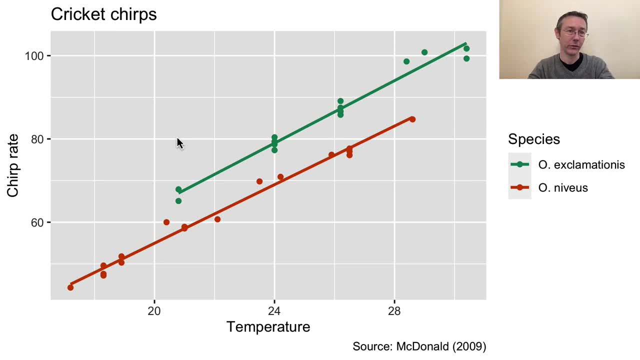 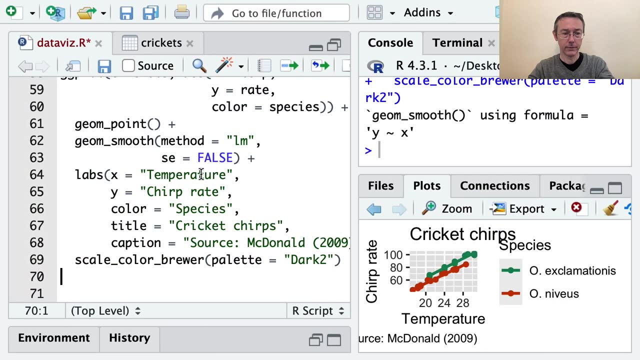 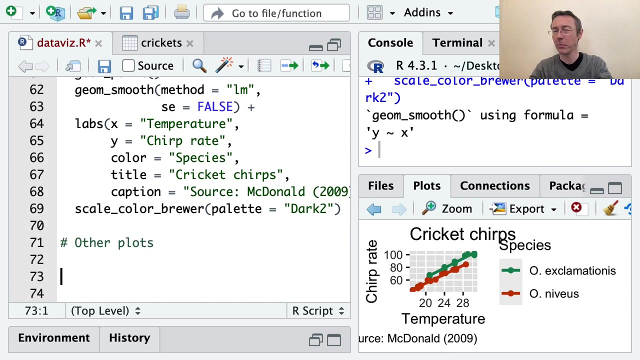 There's. if we were to do a residual plot, we would see that all the diagnostics come up looking very, very good, Wonderful. Let's see here How. about other plots? I did a scatter plot. It's just sort of like an. 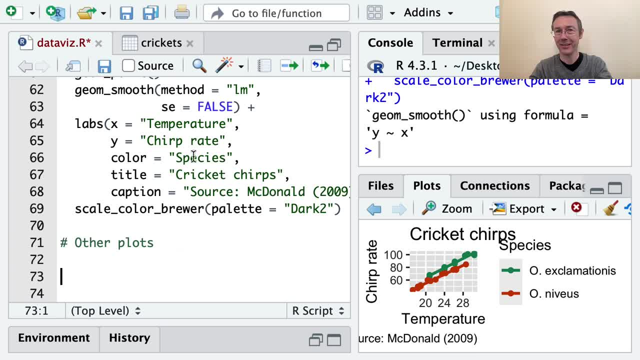 illustration. but there's nothing special about a scatter plot at all. It's a two quantitative variable plot with which you can add a color aesthetic as well. What if you just have a single quantitative variable, Or a single categorical variable, or one of each? These are all different sorts of plots. 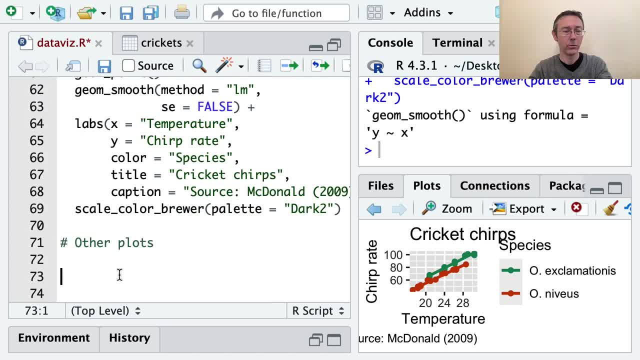 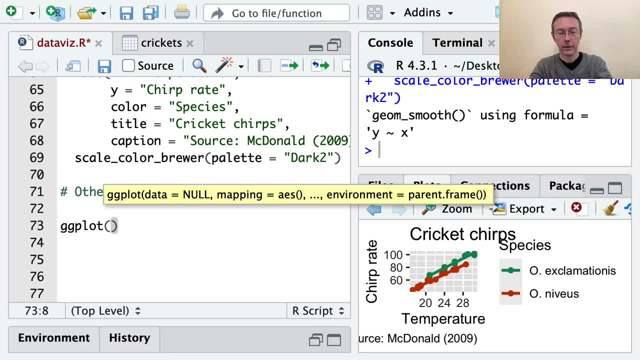 with corresponding different geomes. So let's do a few of these, Let's do, let's get a histogram of the chirp rates. So ggplot crickets. first, I name the dataset AES. I name the variables that I want and where. 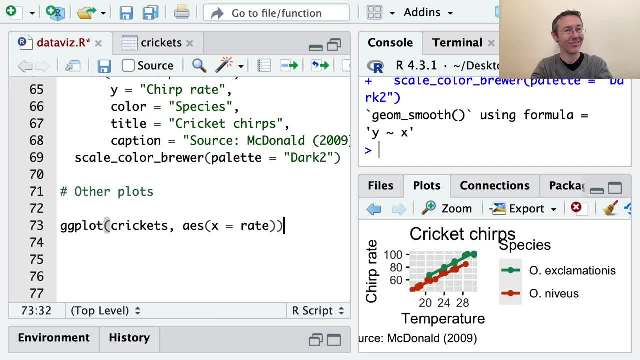 I want them. So in this case, I want chirp rate. In this case, that's all I want. A histogram represents a single quantitative variable with frequencies going on the vertical axis, typically, frequencies being computed just as counts in the data. so really there's only one column being 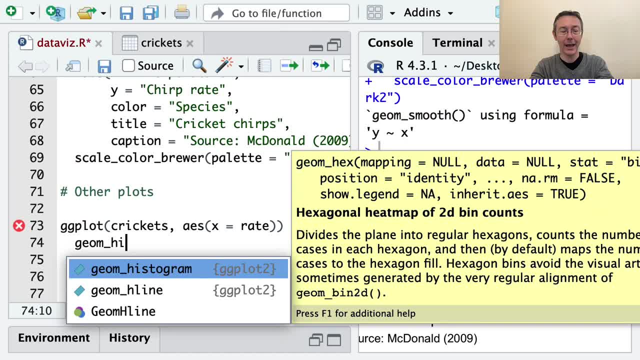 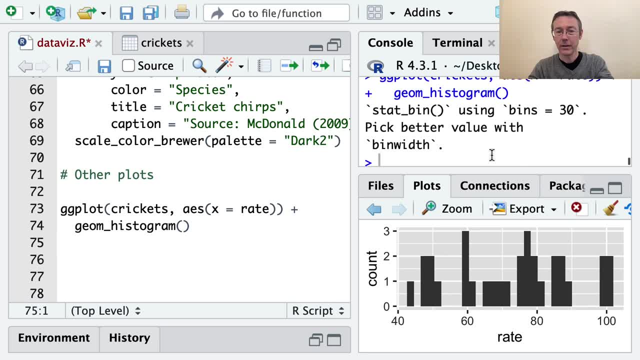 considered here and then to get a histogram. i want to add geo histogram, naturally enough. so there you go, you can see it. the default, as we got in the message here, is to use 30 bins, which isn't a particularly fabulous number. it's intended, i think, to be kind of a default. that will get you. 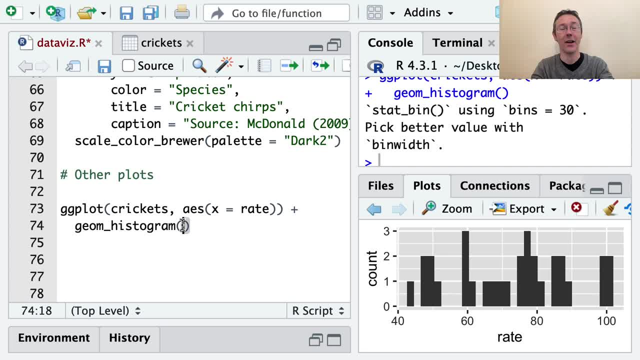 to tinker around. i think good data exploration practice is to try a bunch of different numbers of bins. sometimes the trends you see in a data set will be very different if you're looking at a lot of bins versus a very small number. just for illustration, i will change the bins to 15 here. 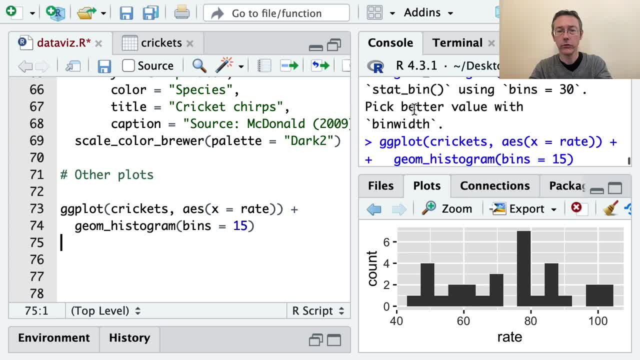 there we go. you can also change how the bins are displayed with bin width. so instead of bins equal 15, i could put bin width equals 5, for instance. all right, lovely, that is for um one quantitative variable. i think this is a good moment to see the strength of the ggplot perspective. the 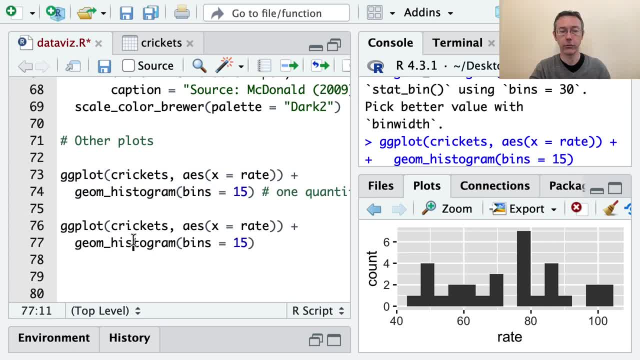 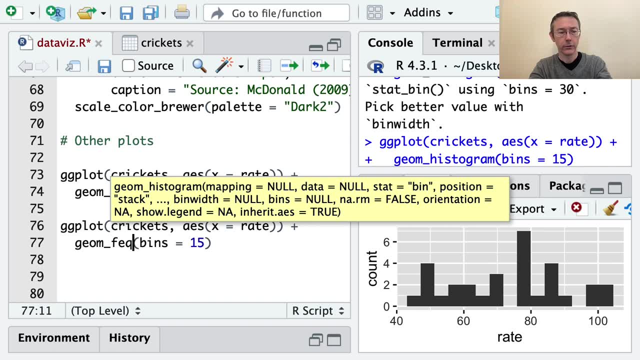 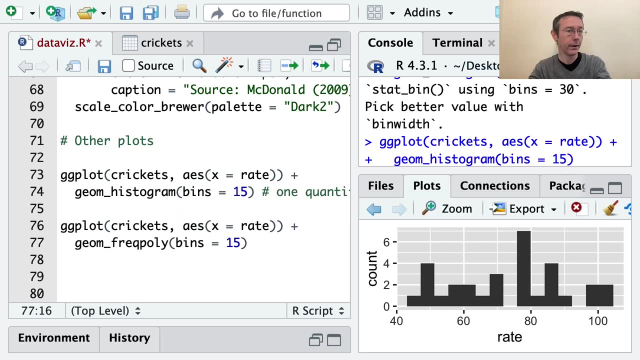 grammar graphics perspective: that histogram should come later in the call, not right up front. let me just change from histogram to freak poly f-r-e-q-p-o-l-y. this is going to give me a frequency polygon and i want you to watch and see how the plot changes, but then also how it doesn't. 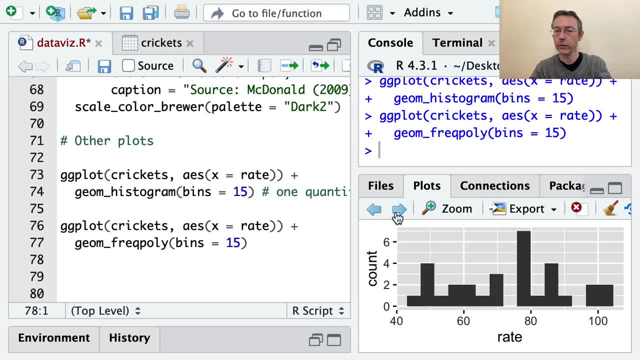 and i'll just do the other one again. can you see how this is exactly the same plot, just represented in a different way? the fundamental feature of this plot is not that it's a frequency polygon or that this one is a histogram. the fundamental feature of the plot is that chirp rate is on the x-axis. 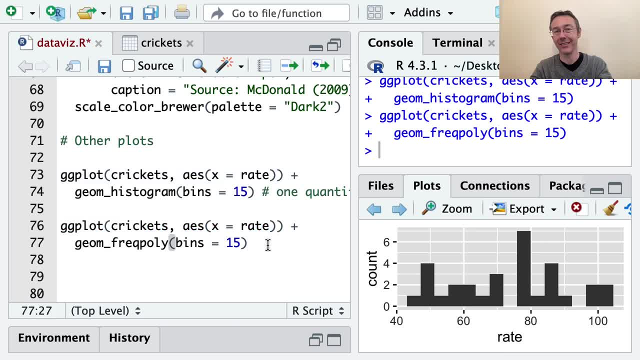 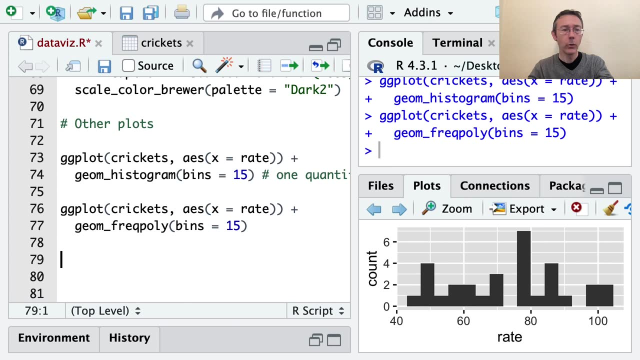 so it makes sense to specify the chirp rate from the data- the crickets data set first and only come back later, and specify a frequency polygon. there are a lot of other single variable geomes that are available to you. i'll talk a tiny bit more about that in just a minute. let's do um a plot. 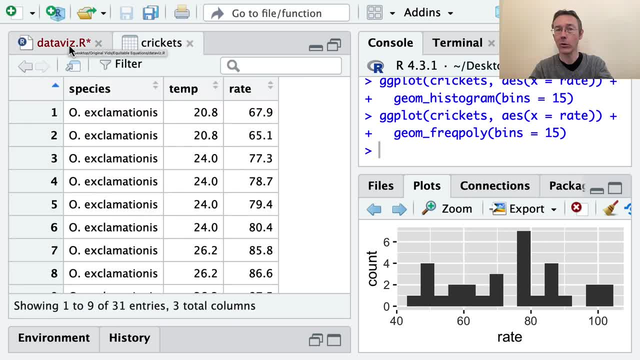 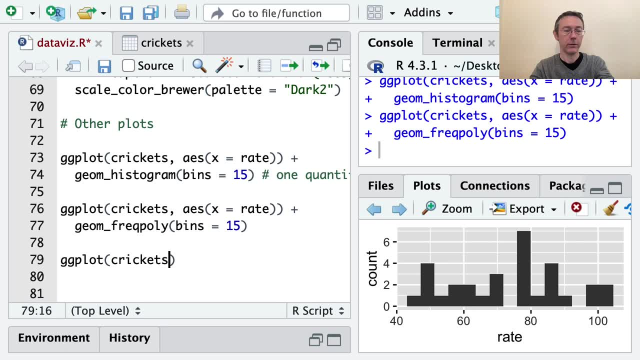 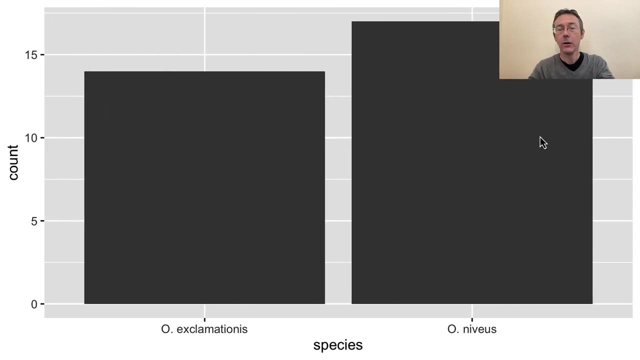 for the species variable. it's a single categorical variable. i want a bar chart, so ggplot crickets, if i can type properly, which is always my challenge, and this time i want my x aesthetic to be species and i want geom bar. there we go. i'll zoom in on that a little bit. you know we can do. 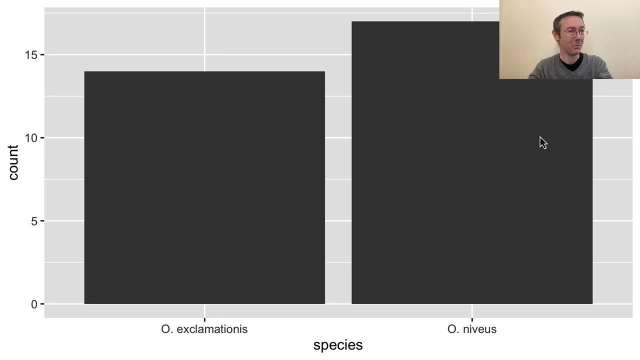 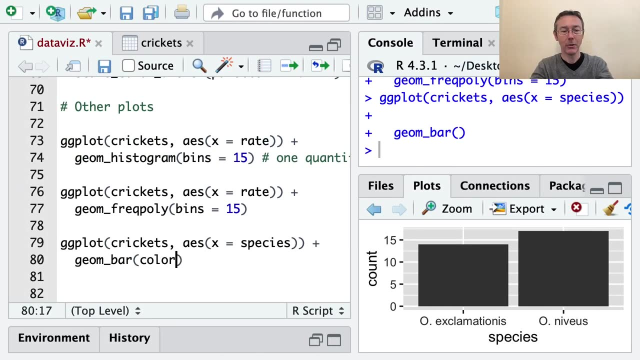 all of our usual things with this. we can change the labels on this, we can put a title, we can add some color. let's actually do that. let's add: uh, how about color equals? i'll start with black. could you see that difference? so color gave me the boundary color. 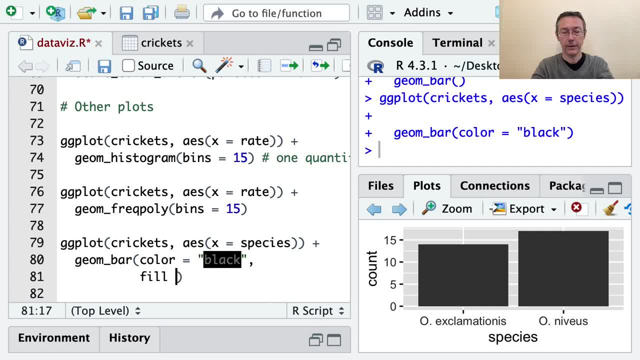 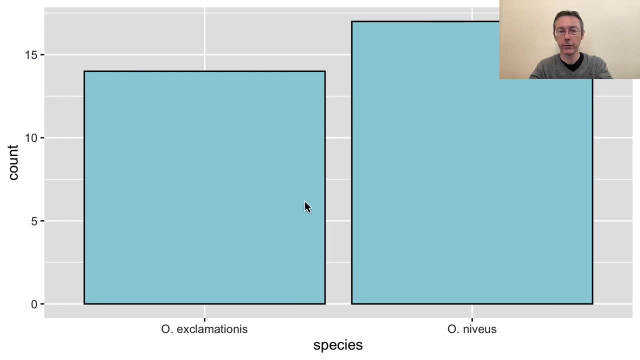 if i want to actually do the inside, i need fill, and so it's fill equals, i don't know. so we've got black on the outside. how about, uh, light blue on the inside? let's give that a try. yeah, that's all right. i'm not sure i love the, the color choices. i'm not a graphic designer. 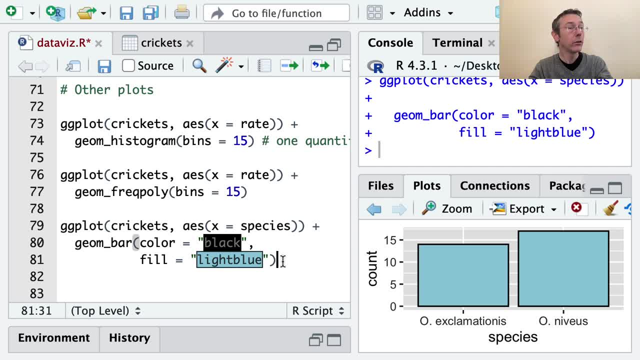 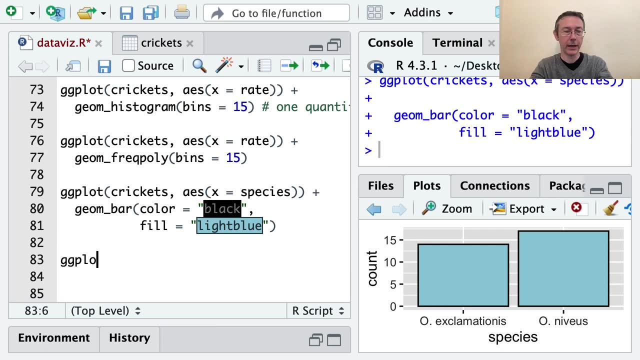 so it's not always perfect in that way. notice that those colors are not being specified by a variable. the colors are being specified just manually. i'm saying: make all the bars light blue with a boundary color of black. now we can have the color specified by a variable, so i'm just retyping. 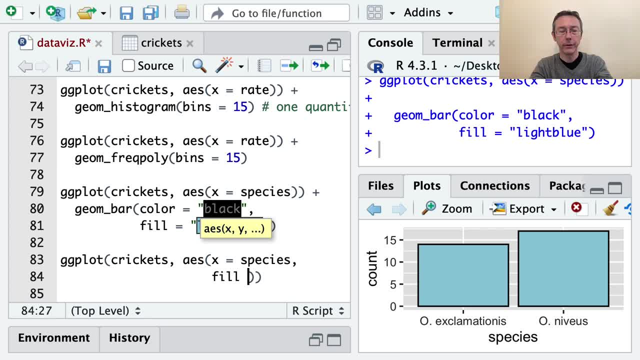 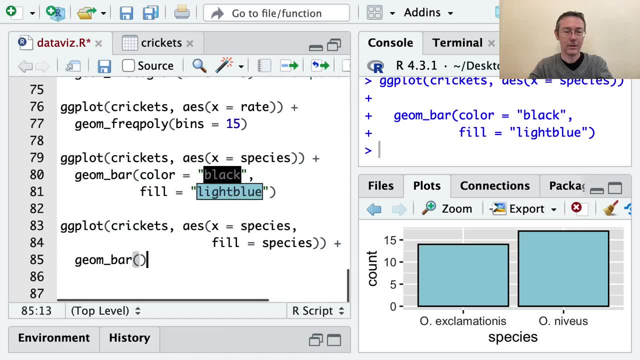 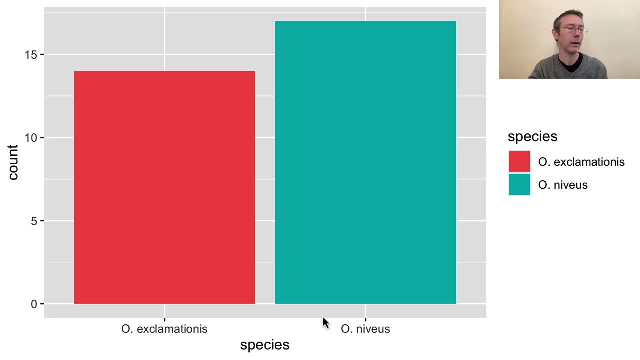 x equals species, so let's make the fill equal to well, species. try and imagine what that's going to do. so this time we have one aesthetic species, but it's being. it's showing up two different ways. species is being communicated on the x-axis as well as with the color aesthetic. so, um, actually, before i do anything else, let me 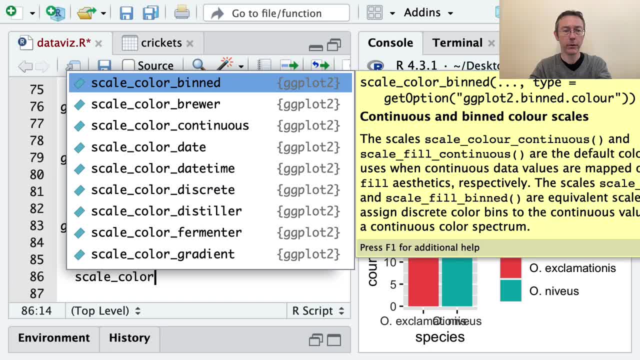 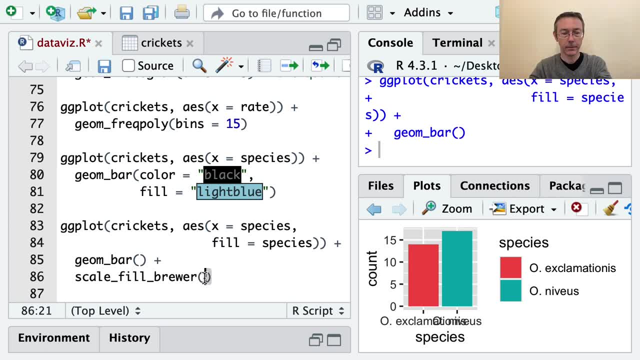 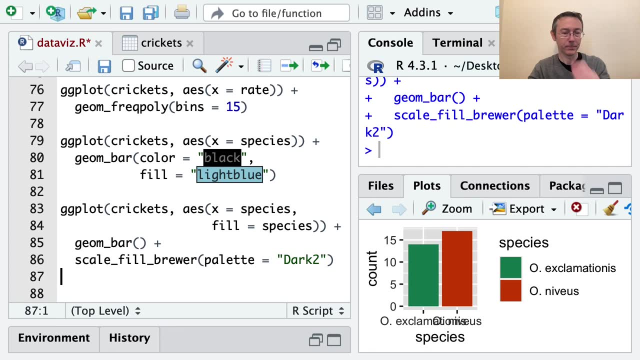 make this a bit more accessible with scale color brewer and actually- wait, it should be scale fill brewer this time, because it's a fill aesthetic and i want palette equals. quote: dark 2, accessibility or bust, okay. so the color is nice. it looks a little bit more professional. we have 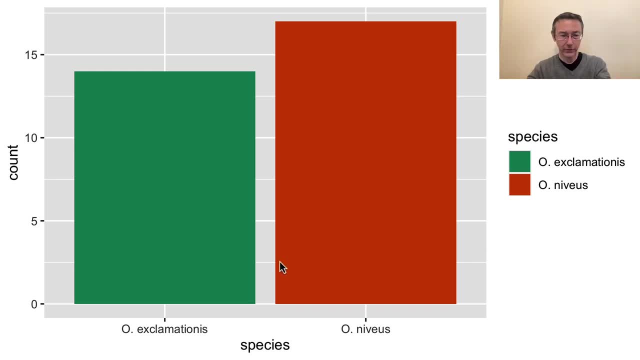 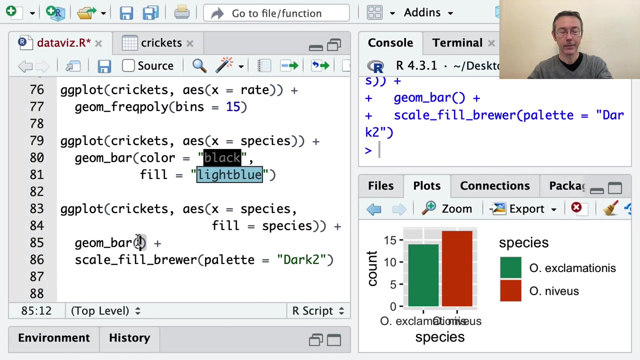 these two different groups with two different colors. the downside is we have the label happening, we have the x-axis as well as the legend. we don't want this legend, honestly. we'd be just as well off without it, probably better. so that's a special property for geom bar and we. 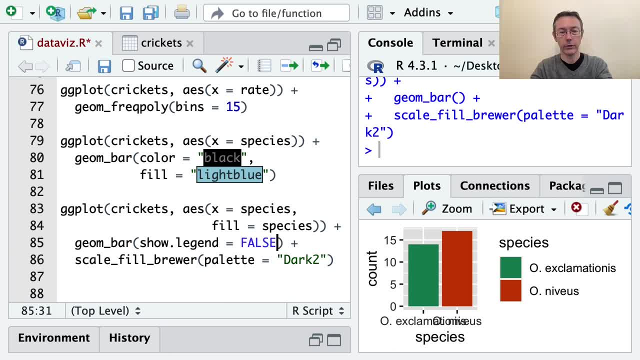 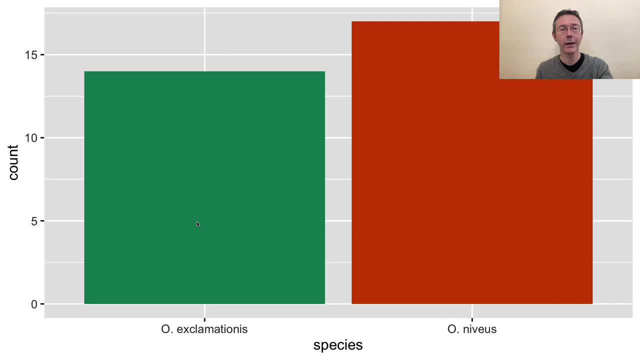 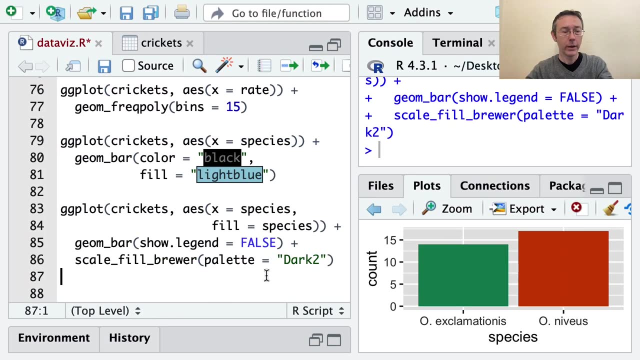 can adjust it with show dot. legend equals false, so don't show the legend. there we go. so now the species variable is being communicated in two different ways, but we only need one label for that. We don't need that extra legend. OK, great, So the bar chart is your default go-to. 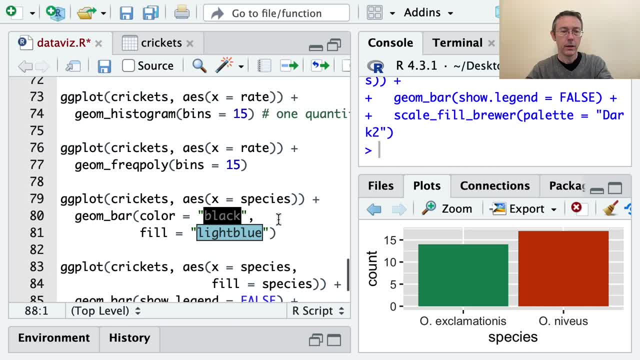 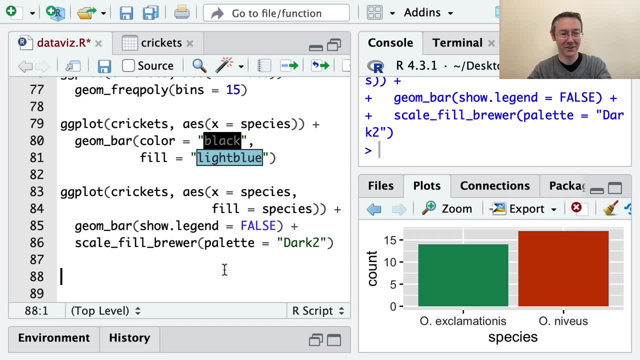 for a single categorical variable. Your histogram is generally your go-to default way of displaying a single quantitative variable. The scatterplot is good for two quantitative variables. The last one I want to show right now is for one quantitative and one categorical variable, And a good way to deal with that is with a boxplot. 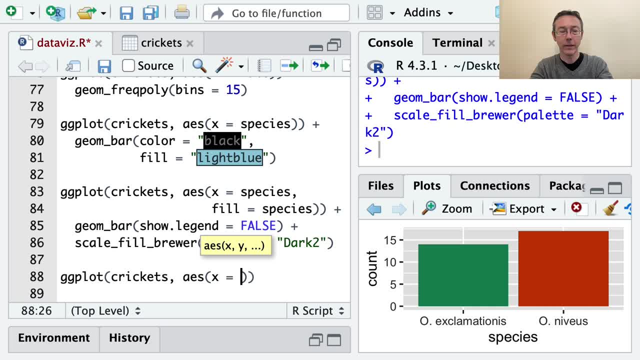 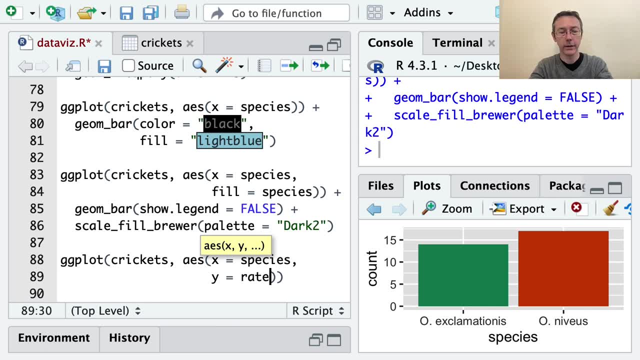 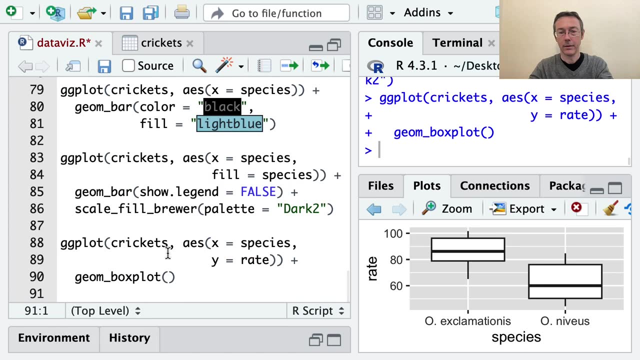 So I'll stick with crickets. On my x-aesthetic, I'm going to put species On my y-axis. for my y-aesthetic I want a rate again And I want a geome boxplot And I'll zoom in on that. 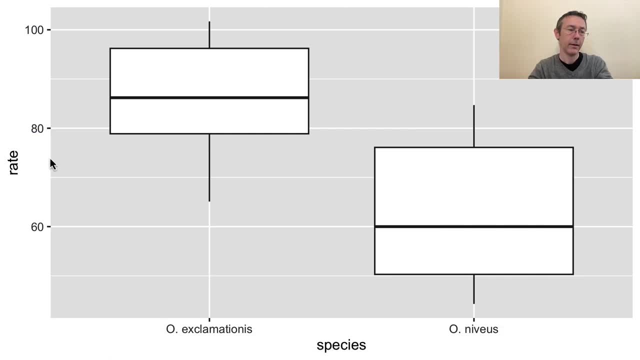 Again, Categorical variable species is going left and right, The quantitative variable rate is going up and down, just as I said in my aesthetics here, And then it's generated a side-by-side boxplot showing the chirp rates for each of these two different groups. 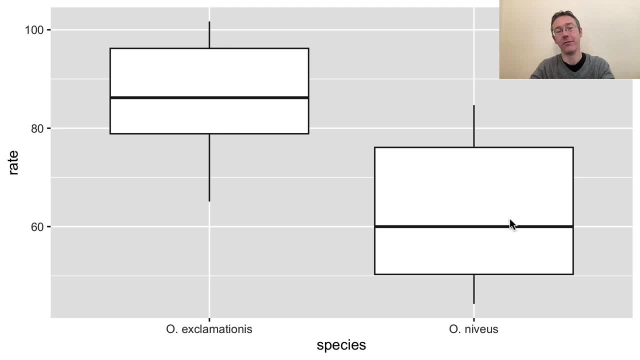 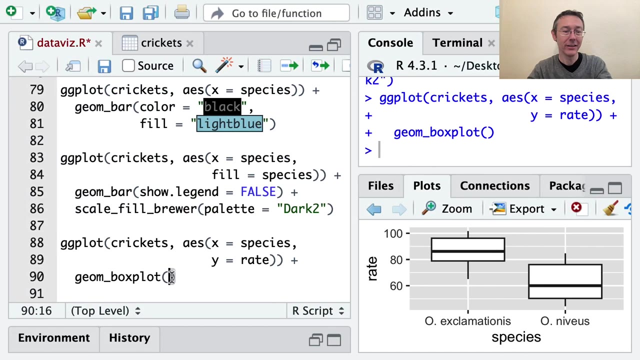 Remember, a boxplot is a visual representation of your five-number summary. So you've got the minimum first quartile, median third quartile and maximum for each of these two sets. You can do things like messing with the color and the fill here. 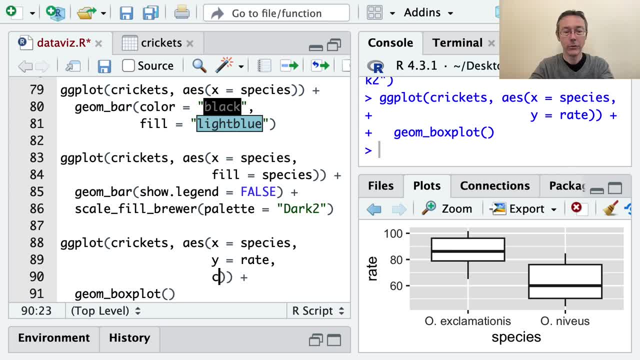 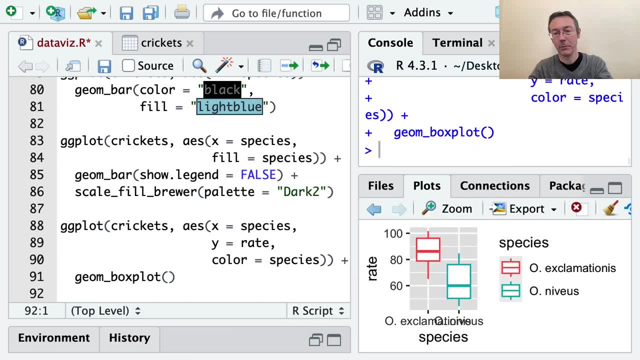 So, for instance, we could do- I don't know how- about color equals species. So this time each of the two will have a different color depending on which species of cricket they are, And I guess I should do my usual stuff. 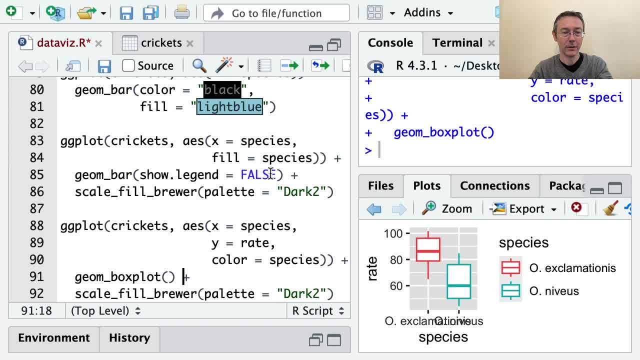 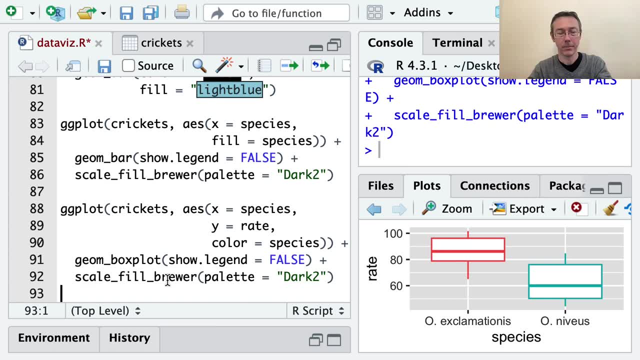 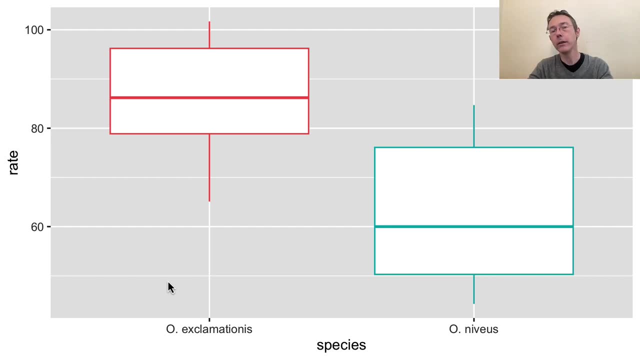 I'll just copy and paste to make that accessible, And I'll also copy and paste: the show legend equals false, so that that's not repeated. OK, great, When you're planning out a data visualization, you should be thinking in terms of which variables you're using. 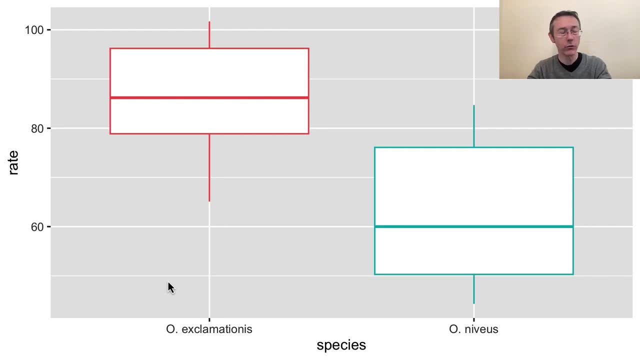 whether they're quantitative or qualitative, And this corresponds very directly to the data question you're asking In this case. I'm interested in a data question relating chirp rates to the different species, Something like: do these two different species have different chirp rates? 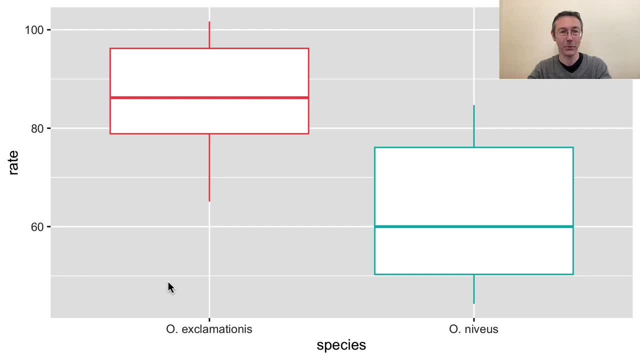 Or do the exclamationists sorry for the pronunciation? do they have a higher chirp rate on average than the nevaeus? And so this visualization helps answer that question. Once you've decided that you have a single quantitative and a single categorical variable, 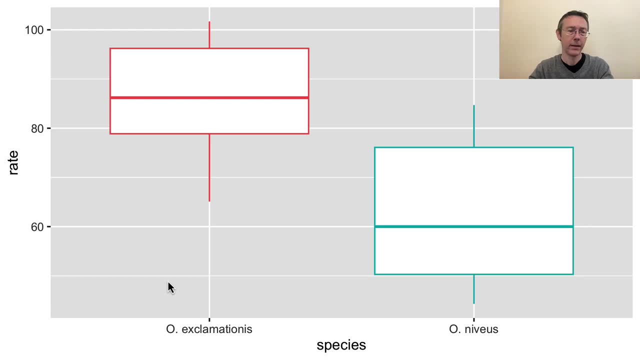 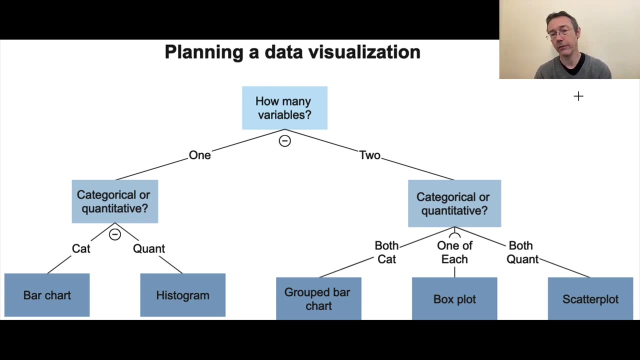 that gives you guidance into what sort of geome you might want to be using. I have a little flow chart that I'll show you And I'll put this up on my GitHub in case you want to download it- When I'm planning a data visualization. 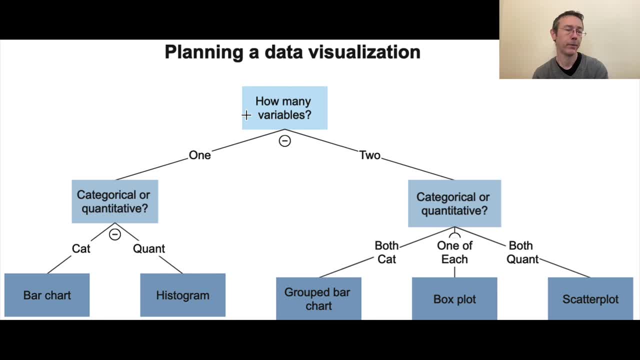 I'm starting by asking: how many of these species do I have? And I'm asking myself how many variables I fundamentally have. Do I have one, two? I'll talk about three in a second. If I have a single variable, I ask myself. 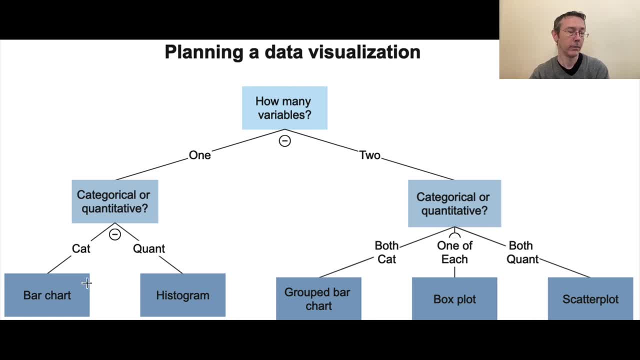 is it categorical or quantitative? If it's categorical, my go-to is a bar chart. If it's quantitative, my go-to is a histogram. Obviously, there's other choices, but these are your most basic and generally the clearest ones that you could pick. 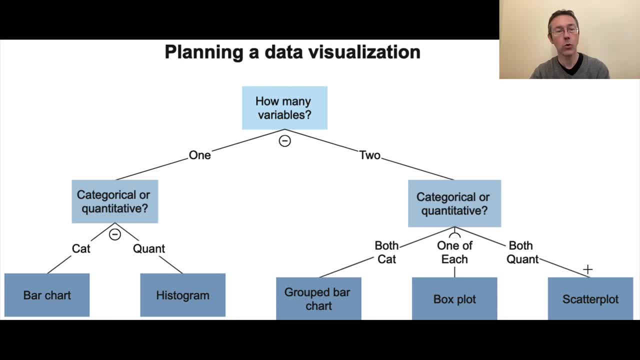 If you have two variables, you can have two quantitative, a scatter plot. You can have one of each, like the box plot that I just showed you, And if you have two categorical variables, you probably want a grouped bar chart. I'm not going to talk about those in this video. 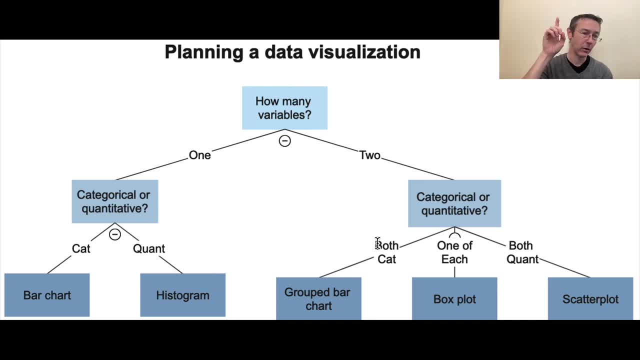 That gets a little bit more complicated. I do have a whole video on that, though. I'll throw a link to that up top. If you want to delve into that, please do. More broadly speaking, if you're looking to do more specialized, more interesting, more potentially. 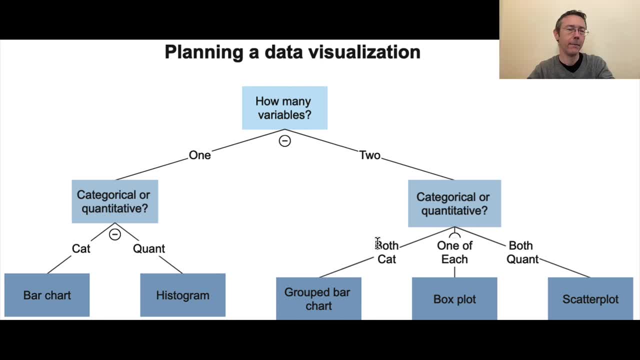 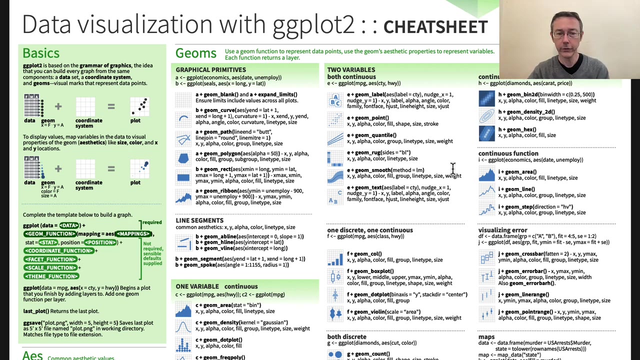 advanced data visualizations And you're curious about how to expand on this flow chart. I'd recommend the ggplot2 cheat sheet that Posit has published. It looks like this. You can find it with a quick Google search In particular, for instance, if you: 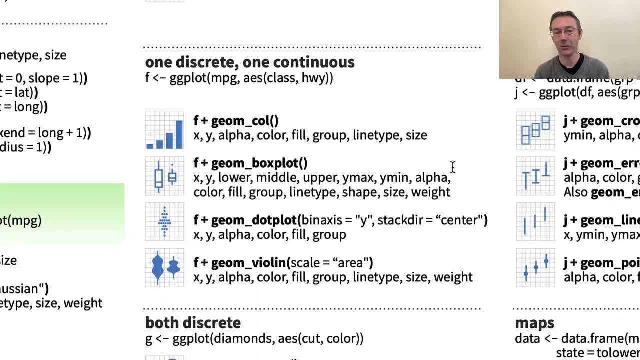 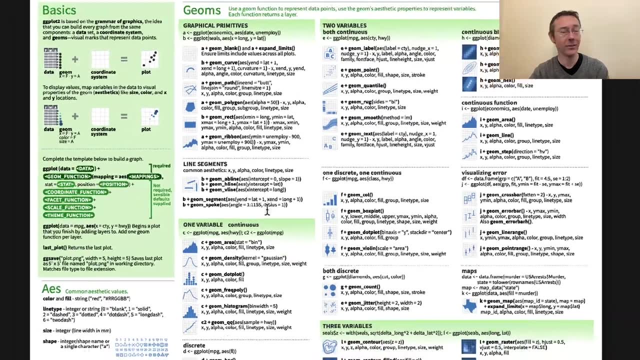 have one discrete and one continuous variable. here are some other options that you might explore, For instance, a violin plot or a certain kind of dot plot here. This is really helpful. You also have a lot of information here about how you can modify things like scales. 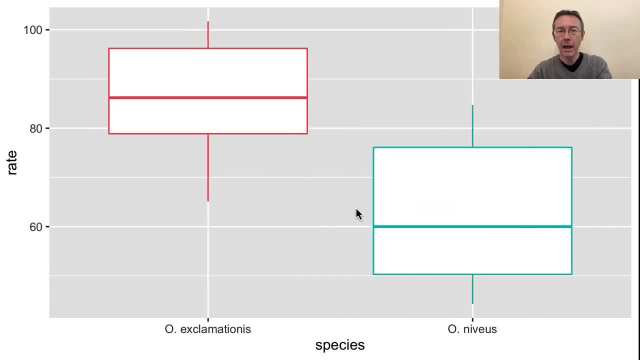 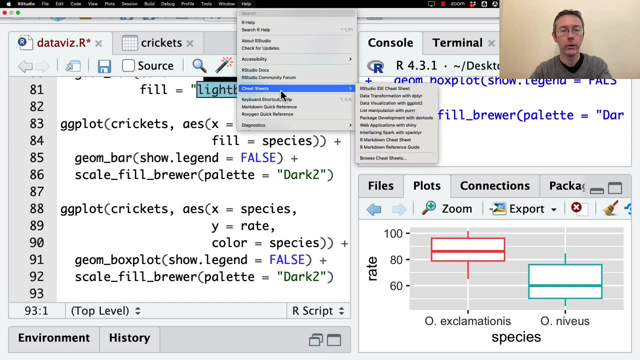 on your visualization. By the way, you don't actually need to Google it, You can go to the Help menu And you'll see in our studio the Help menu has a Cheat Sheets option, So you can go there and you can find the where's the DataVis? 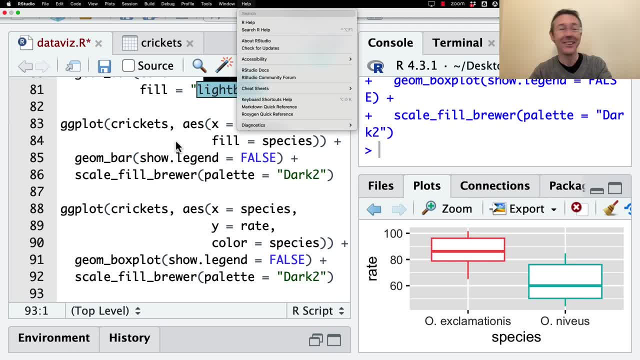 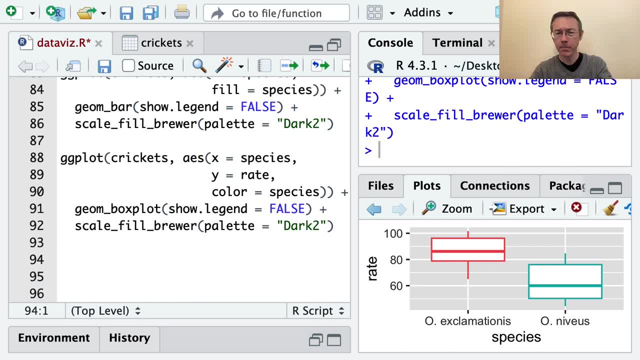 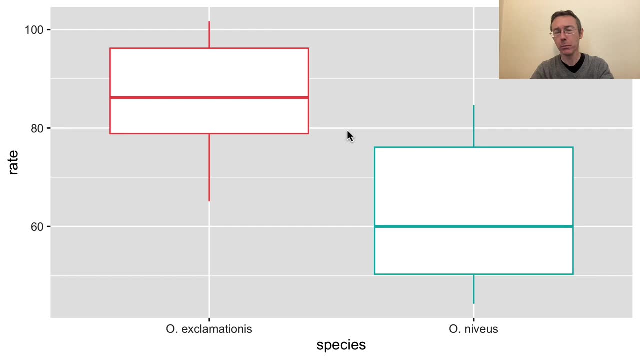 one. There it is, As well as cheat sheets for many other things like data wrangling with dplyr- Great, OK. One other thing I want to do before I'm totally done with this last box plot, And that is with this particular plot. 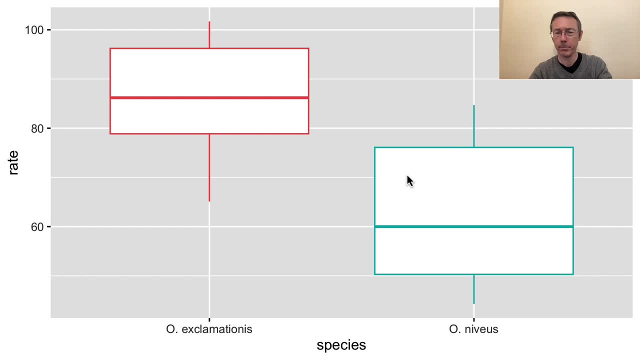 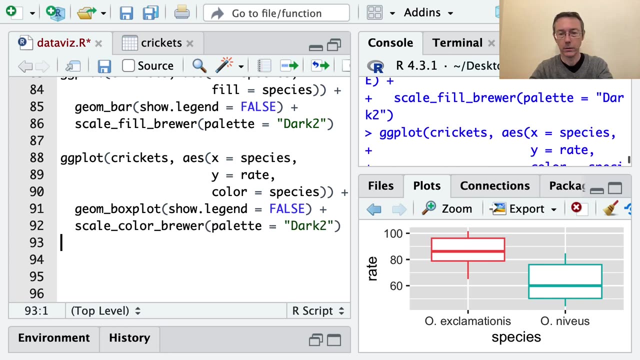 because they're white with the colored boundaries. hey, I thought I changed the color palette. It should be scale color. There we go, OK. Did I have the same issue up here? No, that one's OK, All right. So what I wanted to say is: with these white boxes, 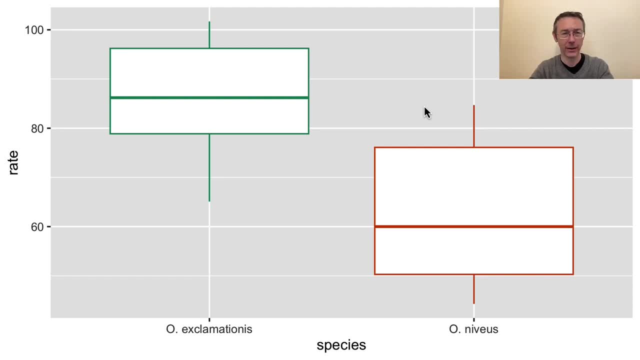 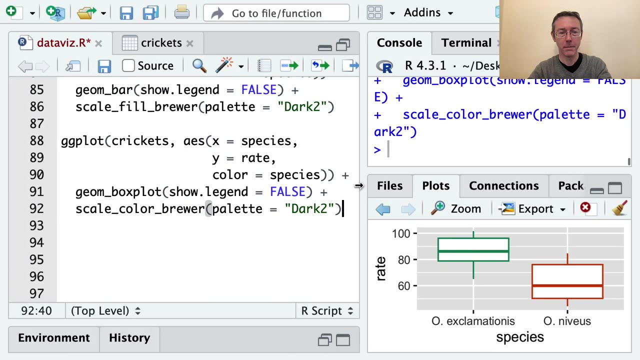 I don't love the gray background. I'm never fully in love with that gray background that ggplot puts in by default. but here in particular We can take that out And in fact I kind of recommend taking it out by adding theme minimal. 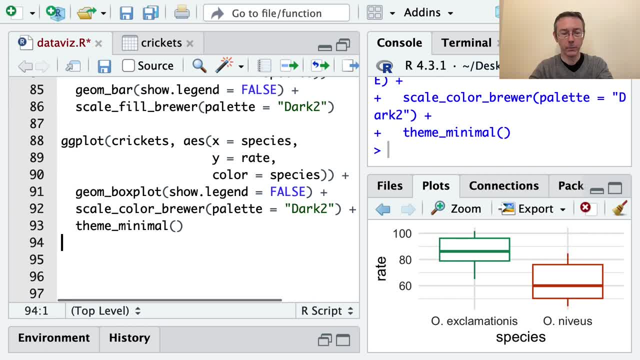 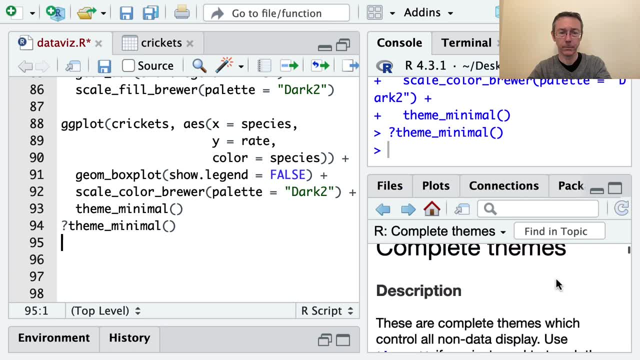 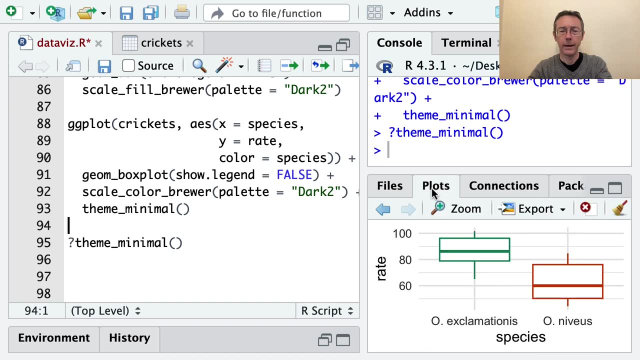 There we go. By the way, there's other themes available to you, And if you do question mark theme minimal, it'll give you in fact some other options for complete themes, So you can explore that on your own time. By the way, it is possible to change things sort of manually. 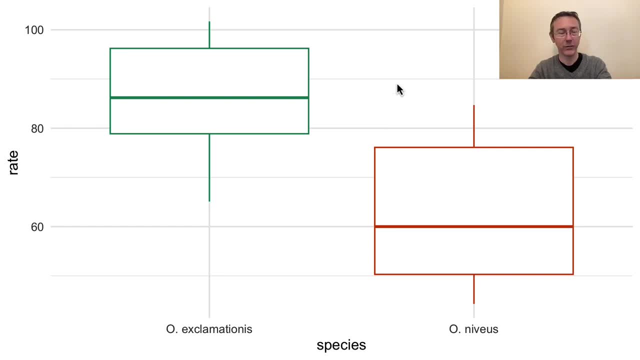 and go in and say, all right, I want to myself specify that I want the background to be yellow and I want these bars to be orange or whatever. In general, I recommend against that, unless you're a pretty advanced user and in particular if you're pretty. 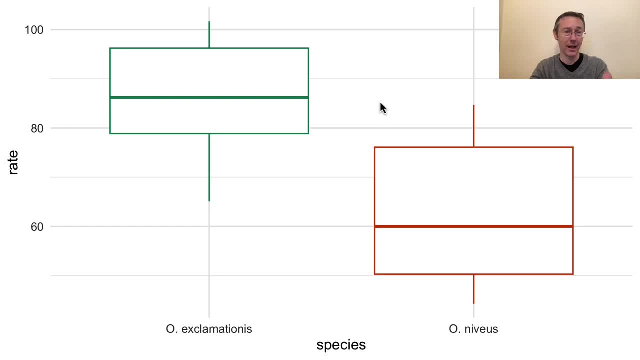 advanced in your understanding of graphic design, Which I'm certainly not. Usually, when beginners with data visualization tinker with that kind of thing, it comes out looking worse than in the predefined themes. Generally I'd say: pick a color palette, use something like theme minimal. 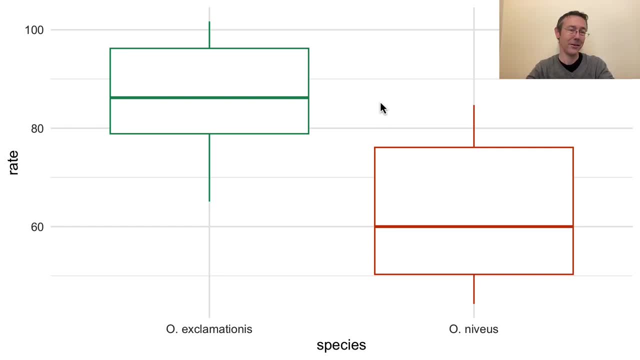 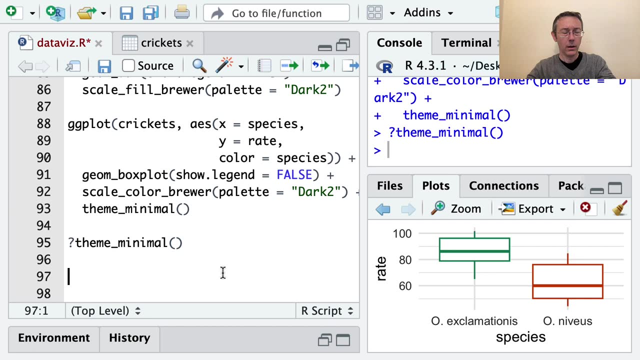 There's a few other good ones, And then just let it go from there, And if you need to do more finely grained things, find a partner that really knows what they're doing in terms of graphic design. The last thing I want to do here is: 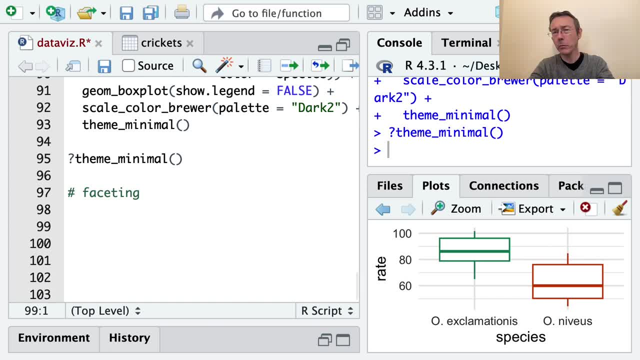 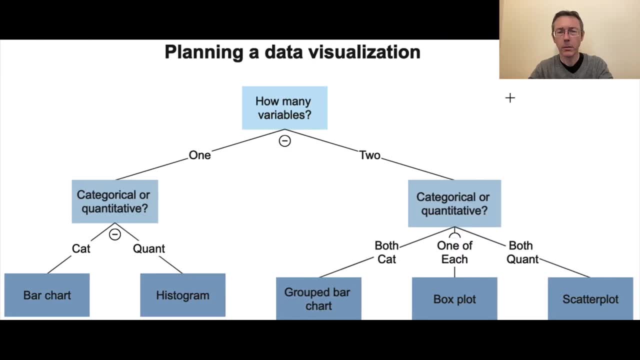 I want to talk about the color aesthetic, And I want to talk about the color aesthetic in general because I think it's really important to understand how color is faceted, So sometimes introducing- oh actually, before I do that, I'm sorry. 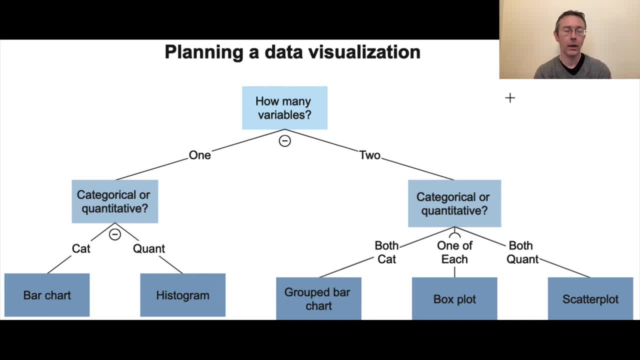 In my planning a data visualization thing. I have two variables here. I didn't talk about three or more, So I want to say something about that really quickly. In general, I only recommend adding a third variable to a data visualization If you can do so pretty clearly using a color aesthetic or something equivalent to a color. 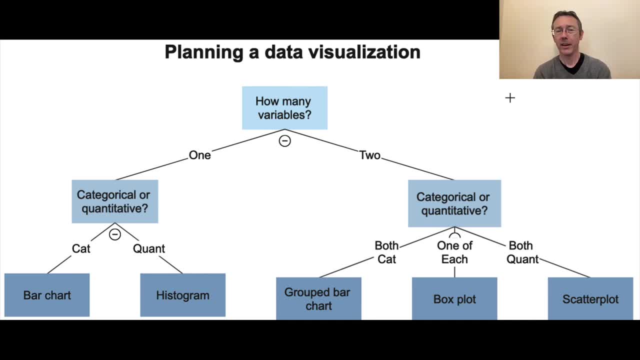 For instance, shape. A lot of times when you start putting in three or four aesthetics, mapping three or four variables to the same plot, the point of the plot becomes lost. Remember, a plot should be communicating a clear data point. Frequently one data point, not many. 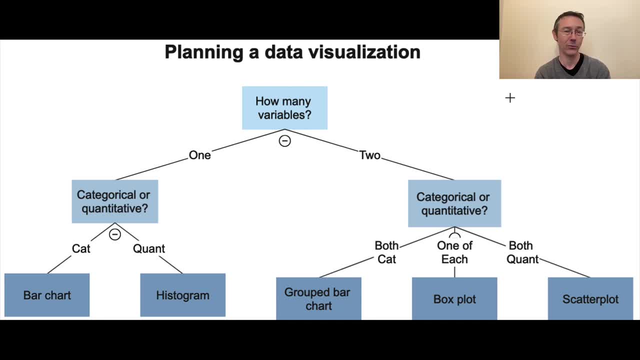 And when you put in three, four or five aesthetics, you start detracting from that And the plot becomes harder to read. So if you've got a scatter plot with two quantitative variables and you want to add a color to it, 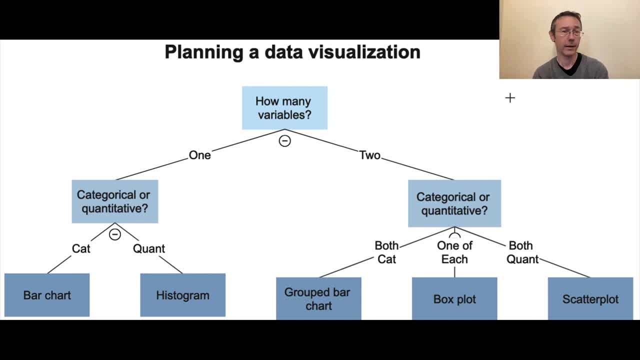 yeah, that's great. Same thing with some of these others that we might have talked about. I don't generally recommend representing a fourth variable. I generally don't recommend trying to represent, for instance, three quantitative variables on the same plot. ggplot2 doesn't support three-dimensional graphs. 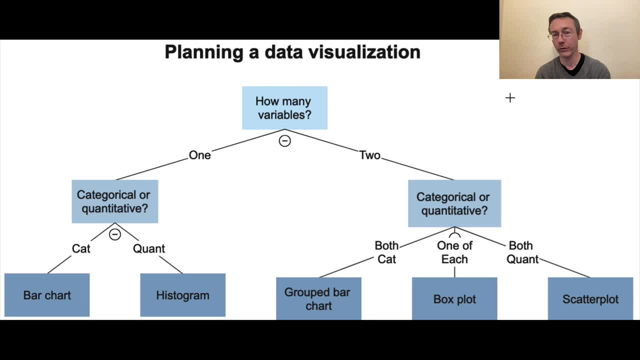 Those sorts of plots are often not considered best data visualization practice Because fundamentally it's a flat image representing three variables, which is relying on optical illusion. That can get deceptive or misleading very easily. So I would discourage you from doing a three-dimensional plot unless you just want something pretty. 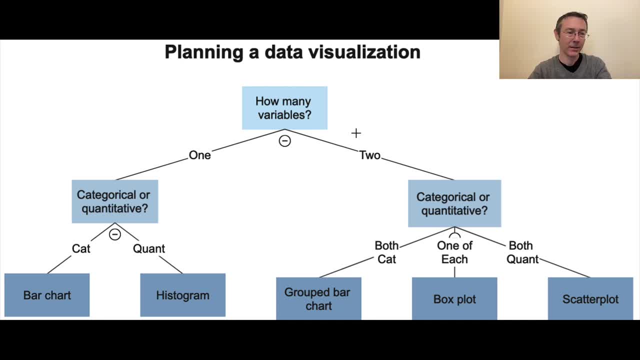 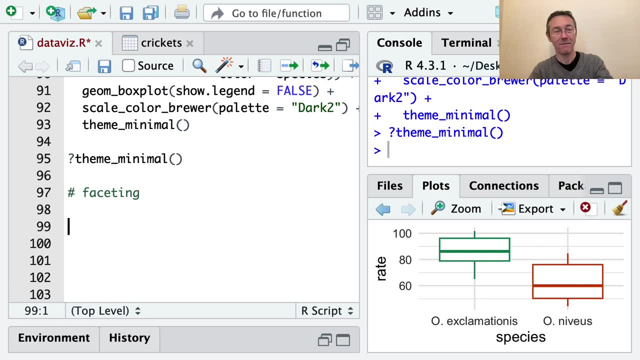 that's not really supposed to be fully telling a data story. There's exceptions to that, like every rule, but that's my general, my general thing. Okay, now for real faceting. So I think the point of faceting is clearest if we try and do, say chirp rate. 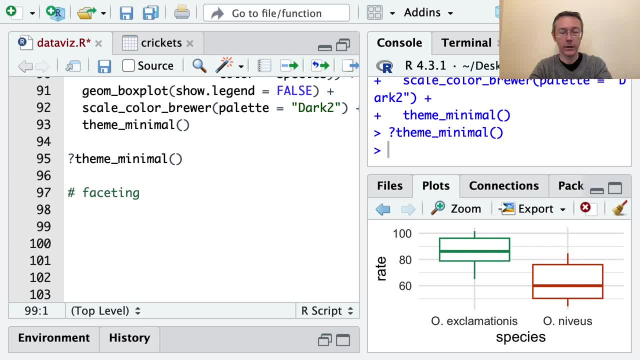 Okay, So we use the three-dimensional plot to do one awesome thing, which is just try and get this thing broken down by species in a histogram. So let me show you that I want to do ggplot crickets. a no i at the beginning of crickets. 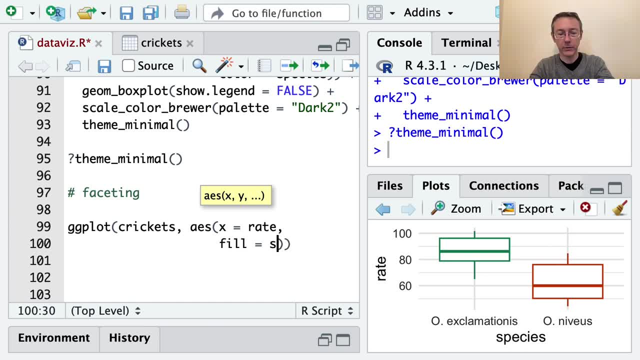 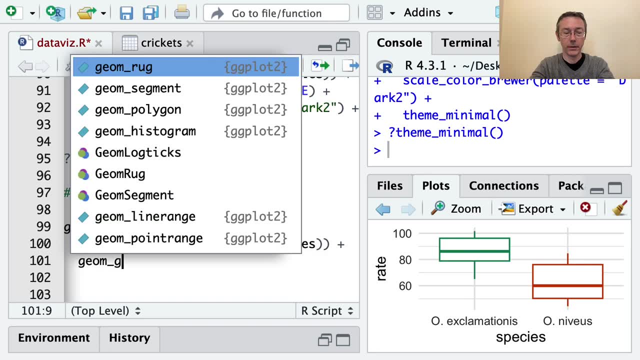 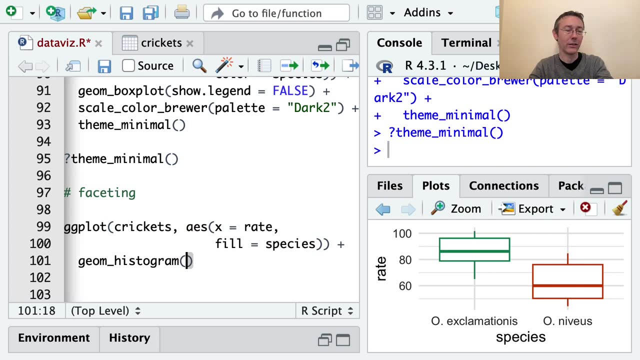 On the x-axis, I want to put rate and I want to fill according to species. So basically, I want to add this categorical variable in to my histogram And this is a valid plot. but I think, at least for me, it's not attractive and it's not going to be overly helpful. 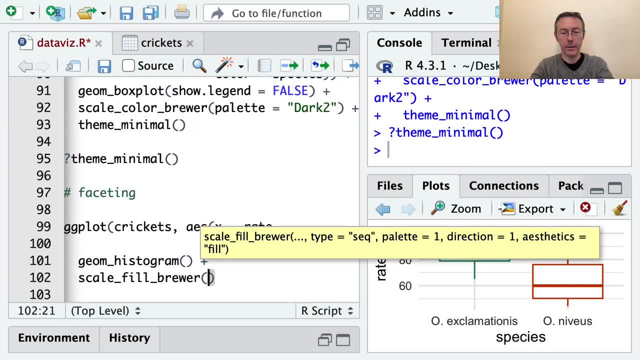 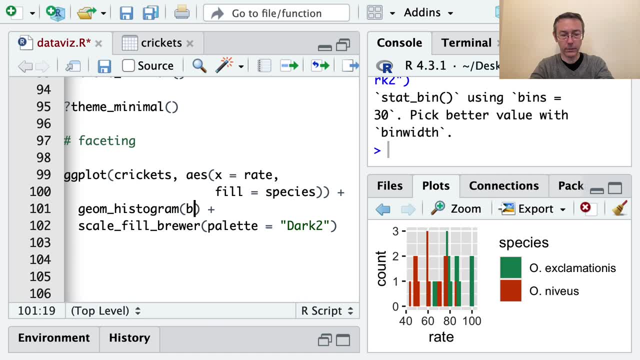 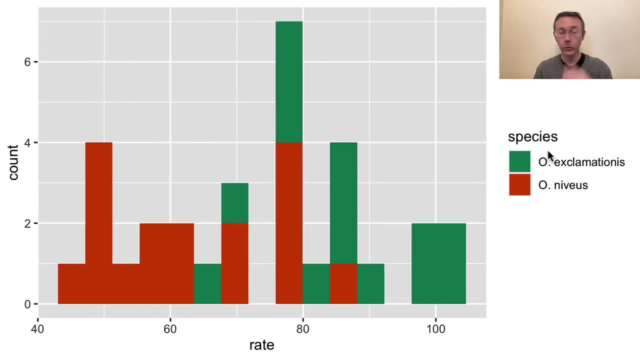 While I'm at it, I'm going to put in a scale fill brewer Palette equals dark2, just out of habit, And let's do 15 bins like we did before. Okay, so it did what we asked. It gave us this histogram with rate on the x-axis, colored by species. 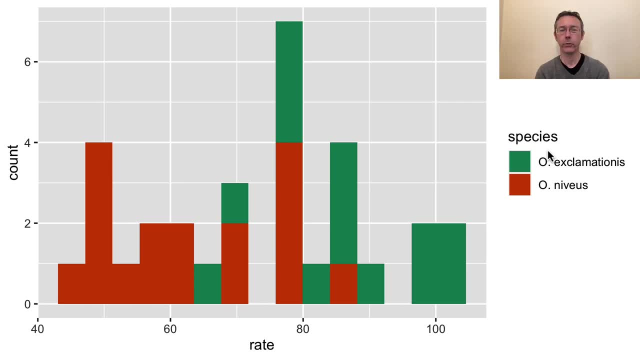 But it's not the easiest thing to interpret. It sort of stacked the exclamationesses on top of the nevaeuses, And here you can kind of tell that the exclamationesses have higher chirp rates. but it's not the most clear plot ever. 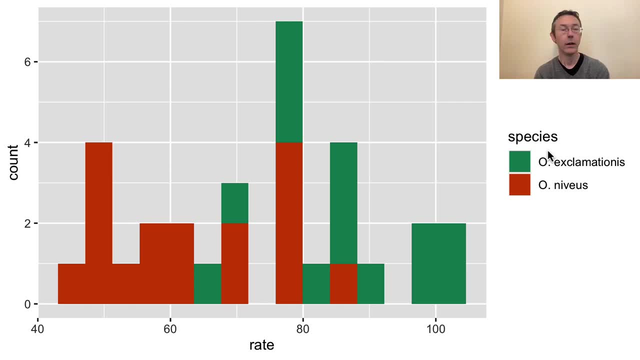 And if you have three, four, five categories, this can get really, really ugly. Honestly, the better way to describe this data and these two variables is with side-by-side, or plots that are right on top of each other. Separate plots for exclamationess and for nevaeus. 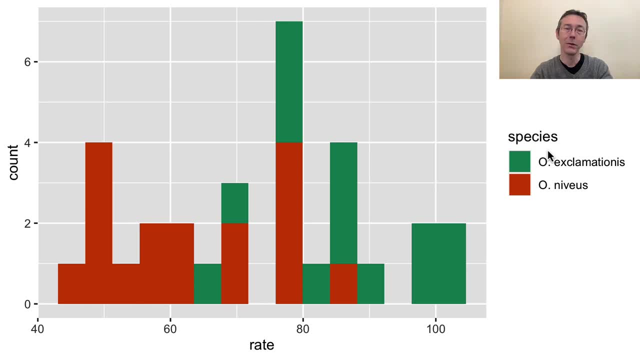 Now the more complicated way to do this would be to break the data set down into two separate data sets and make two separate plots. It's a lot of work, it's repetitive and there's some technical problems with that as well. For instance, there's no guarantee that the scales 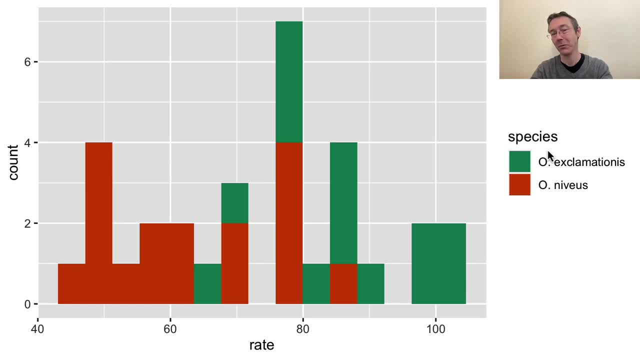 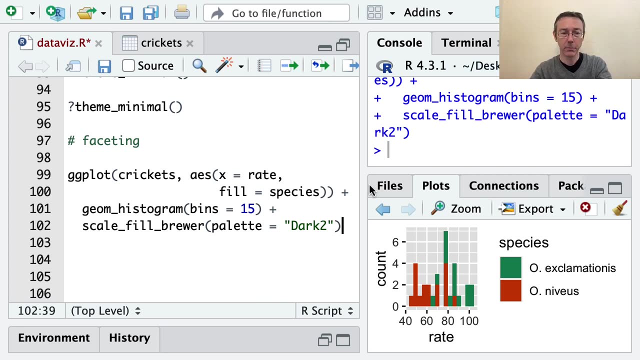 The scales and the two plots will be the same, and so you might not necessarily want to put them side-by-side, even if you had them. The best way forward here, and for the moment I will just take out the species aesthetic, the fill species aesthetic. 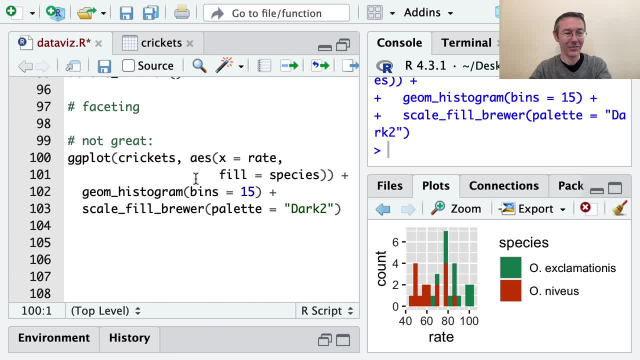 Let me just make a note for the saved file that that's not great. So the first thing I'm going to do is take out that aesthetic. So I want still to do a histogram of rate And I will stick with 15 bins. 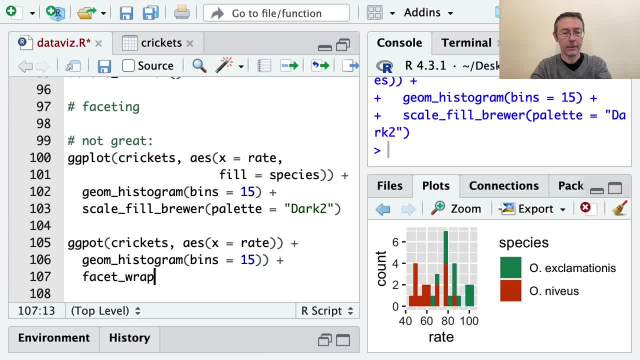 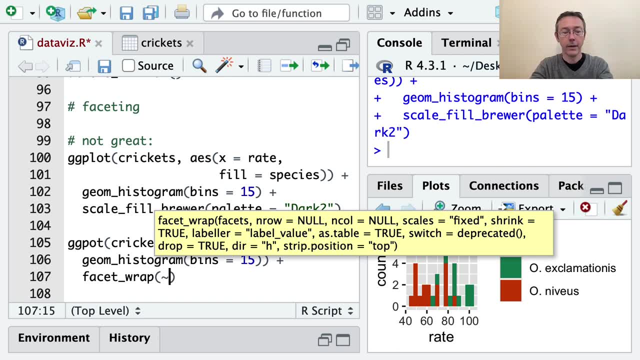 And this time I want to do a facet wrap And this is saying: just give me a plot for every different value of the categorical variable I'm going to specify next. And the variable I want is species- Notice this syntax: tilde species. 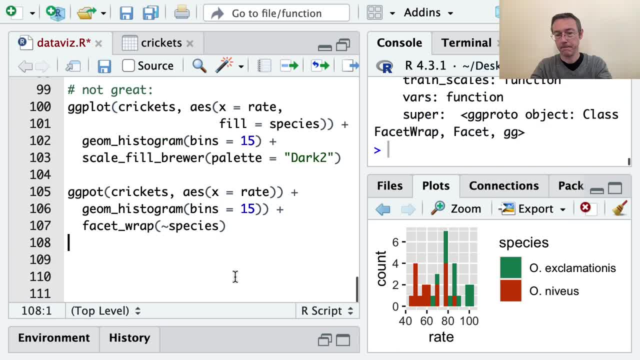 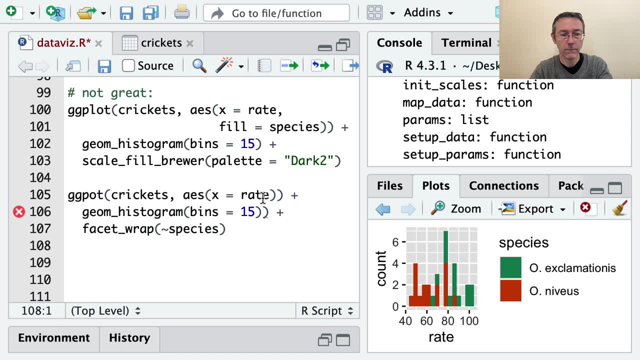 So basically wrap it by species, And I seem to have made a mistake here. Let's see here what is it? Where's my plot? Where's my function? Where's my mess up? It doesn't like my facet wrap. 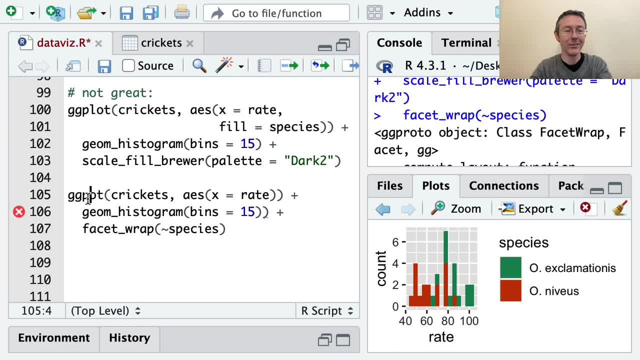 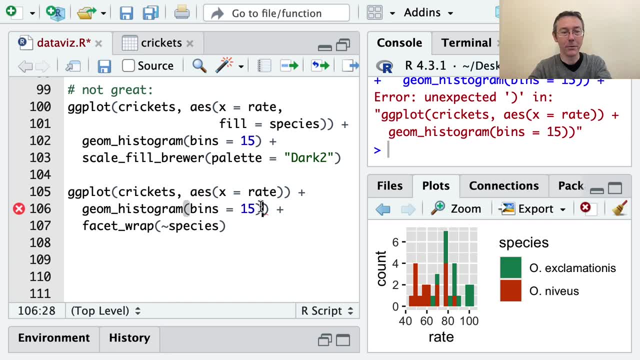 Facet underscore: wrap by species. Oh, it's ggplot is my problem. I just literally misspelled ggplot And now it says I have an extra parentheses here. There we go, There we go, There we go, OK. 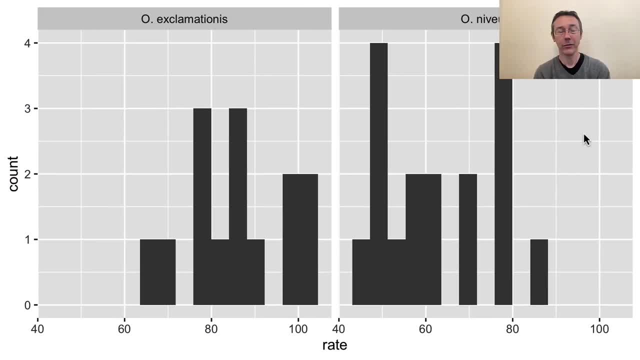 Finally we have it where we would like it. OK, So now we have side by side plots for these two different species of crickets. Notice that the scale for counts is the same on both, even though the counts for the bins for the exclamationesses. 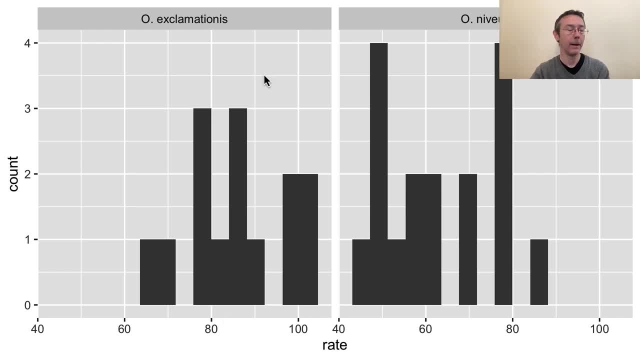 only go up to three. If we had made the plot separately, the scale would have been different. here They're the same And that makes it easier to compare the two side by side. Similarly, for rate they both go from about 40 to maybe 110 or something. 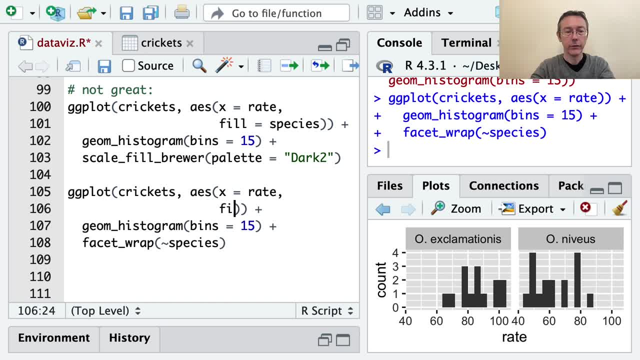 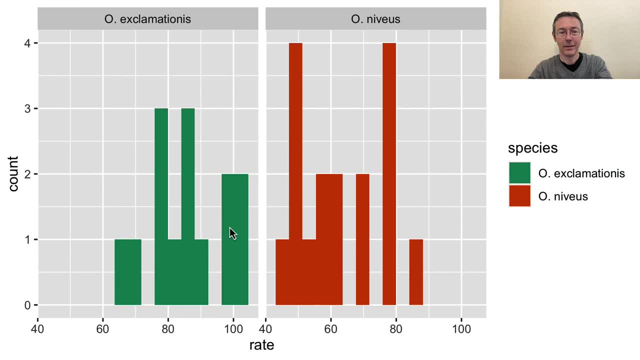 All right, Let's add in some color. Let's do it the same way as before. Let's add in a fill- aesthetic, Let's fill it by species, And if I'm going to do that, I should copy and paste my colorblind, friendly palette, like so: